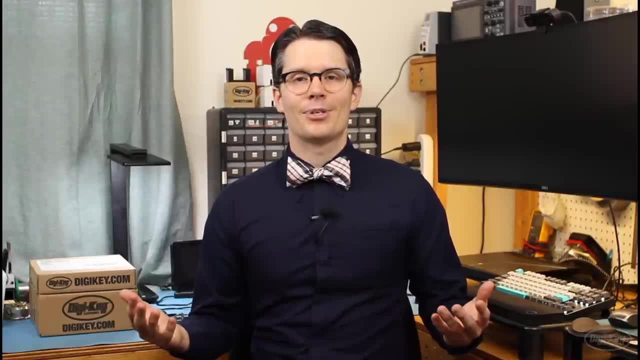 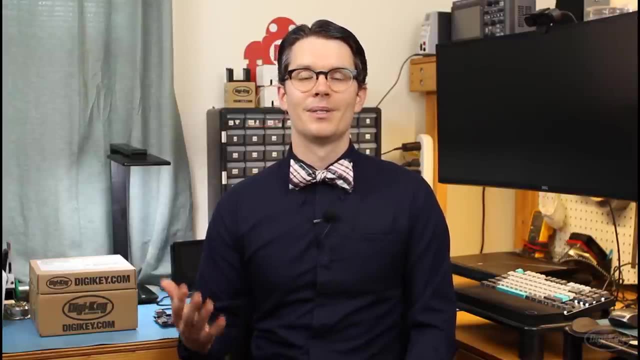 system for embedded devices. Over the next few episodes, I'm going to talk about why you might want to use Linux in an embedded device and show you how to build your own custom Linux distribution. I recommend having some experience with Linux before tackling these projects. 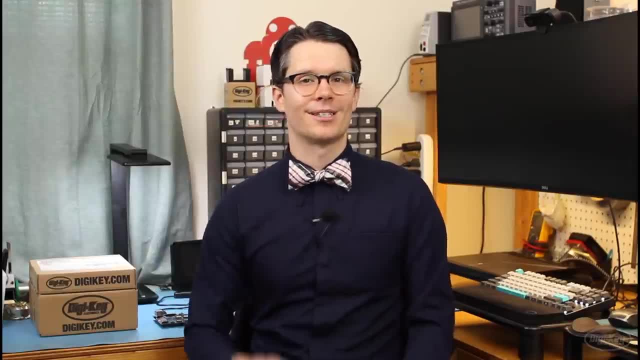 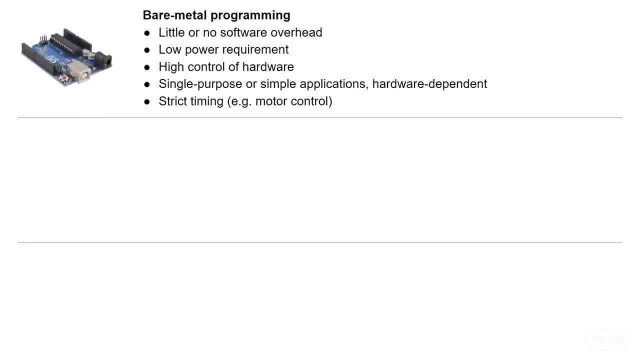 and I'll see you next time. Bye, As we'll be using the command line quite a bit throughout the series. Let's get started. The first question you might have is: why use embedded Linux at all? Let's review some options for embedded development. First is bare metal programming. This is something you might do on. 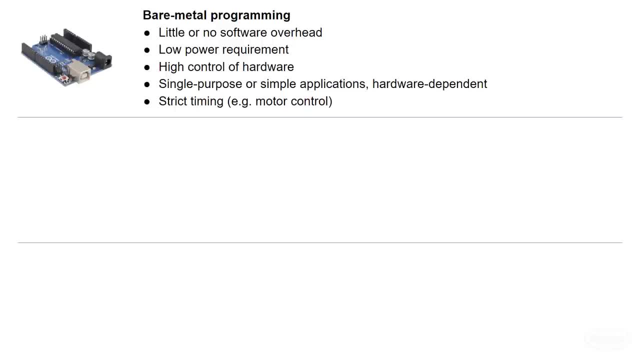 eight, 16 and some 32 bit microcontrollers, and many of them can be very inexpensive Because you can take a little bit of your time and spend a lot of your time on it. you might want to take a little bit of your time and spend a lot of your time on it, But if you want to tailor your code to 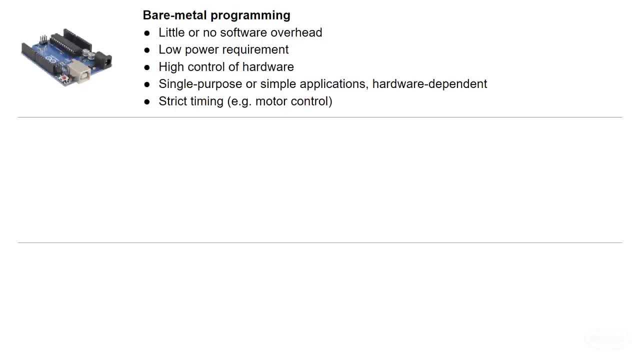 a microcontroller. it often means you can write very efficient code with little or no overhead. You also get direct control of connected hardware. Direct control of hardware often means flipping bits in registers, so your code will not be very portable as it will only run on that particular 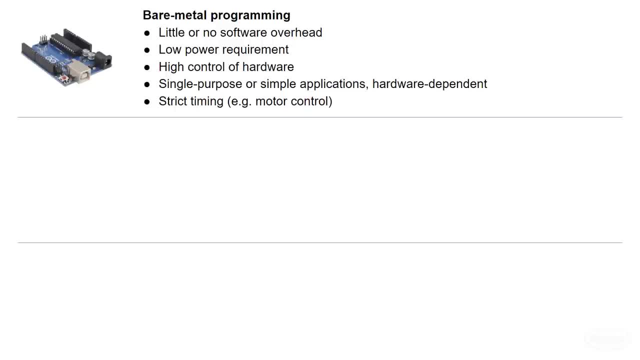 microcontroller family. Without a lot of overhead, you have the option of using low power microcontrollers to get the job done. So this approach is best for single purpose or simple applications and for times when you need strict timing, such as controlling motors or 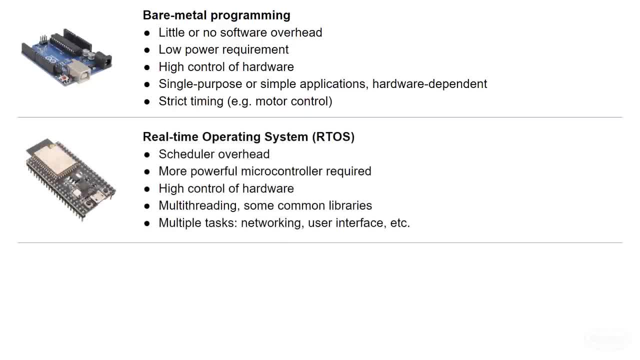 LEDs. Next up is real-time operating systems. These include a scheduler that's almost always running in the background, so there's some overhead in your program. Because of that overhead, it usually means a more powerful microcontroller is required. Some RTOS vendors. 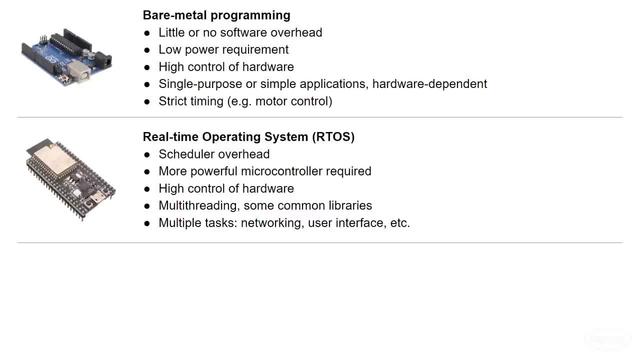 provide support packages for popular microcontrollers, which can include things like library microcontrollers, microcontrollers, microcontrollers, microcontrollers, microcontrollers, libraries and drivers that can make your code more portable. among the supported microcontrollers, You still have the option of high-level control of the hardware, as you can still directly flip. 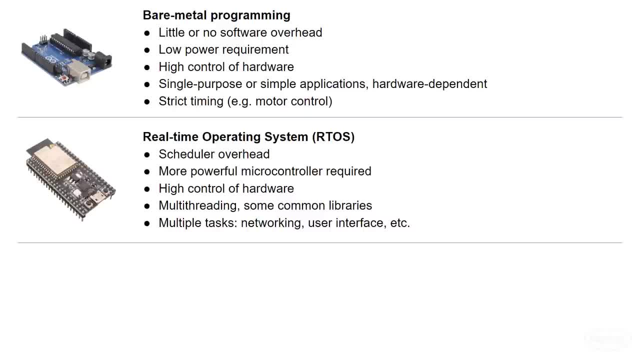 bits in registers, but it might make for less portable code. Having a scheduler opens up the possibility of multi-threading That allows you to run several tasks concurrently, which is useful for things like networking and user interfaces. Additionally, you can still meet strict timing. deadlines with a hard drive. This allows you to run multiple tasks concurrently, which is useful for things like networking and user interfaces. Additionally, you can still meet strict timing deadlines with a hard drive. This allows you to run multiple tasks concurrently, which is useful for things like networking and user interfaces. Additionally, you can still meet strict timing deadlines with a hard real-time. 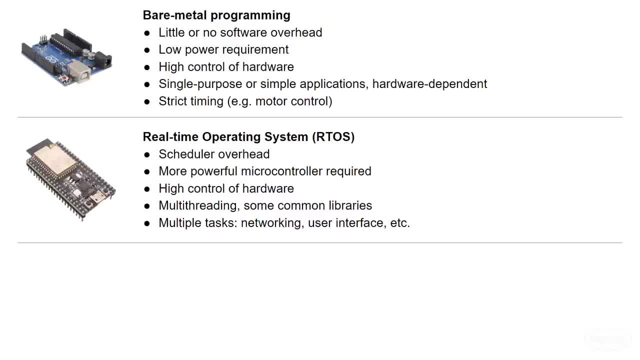 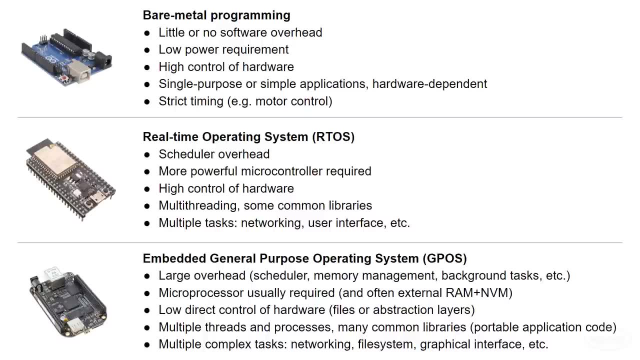 operating system or through hardware timers. Finally, we get to embedded general-purpose operating systems like embedded Linux. Note that running such an operating system requires essentially a full tiny computer, as there is a huge amount of overhead, such as a scheduler, memory management and a variety of background tasks that need to run. 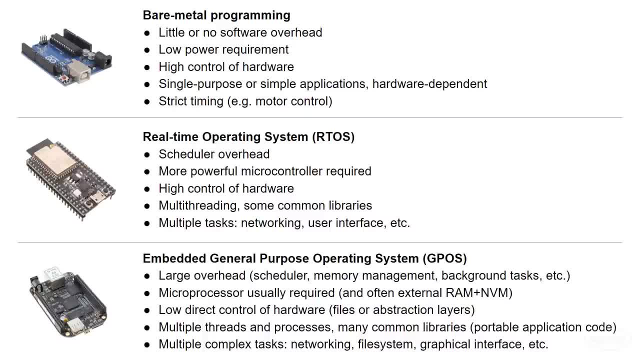 You'll almost always need to move to a more powerful microprocessor and have access to external RAM and non-volatile memory like an SD card. The good news is that you have access to a very fast CPU in the hundreds of megahertz or gigahertz and lots of memory sometimes. 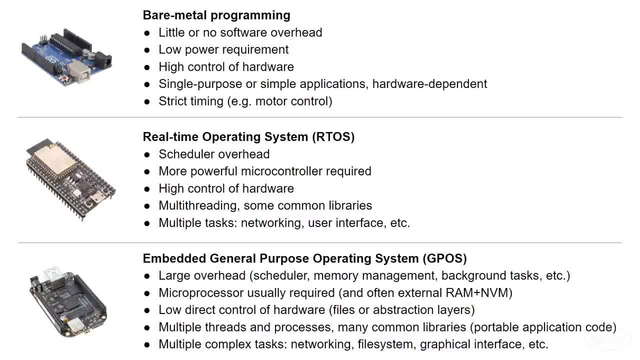 gigabytes. Some applications like video, audio games and some AI require this much power, so you sometimes don't have a choice. These operating systems often abstract away much of the low-level hardware control, so you're working with files, drivers and libraries instead of with registers. However, because of the popularity of operating 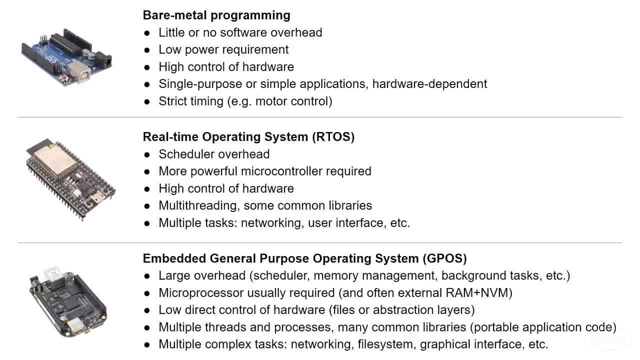 systems like Linux, you can often find vendor or community-supported libraries to help you out. This means you can write very portable code that will work on different embedded Linux boards, and it might also save you development time if you don't have to learn the details of a particular 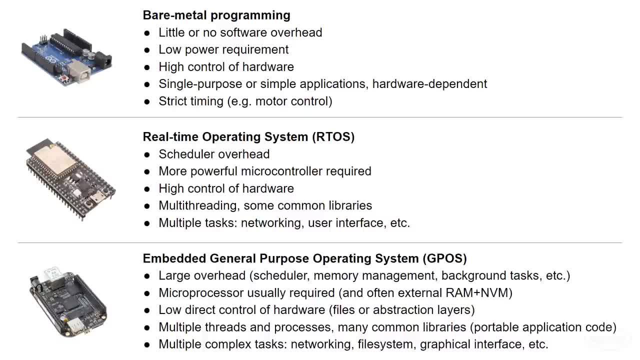 hardware architecture. It also gives you access to high-level languages like Python and Java that you might not have with the other two options. Such operating systems allow you to concurrently run many different threads and processes, and they often give you access to advanced features like networking, file systems and more complex user interfaces. However, because 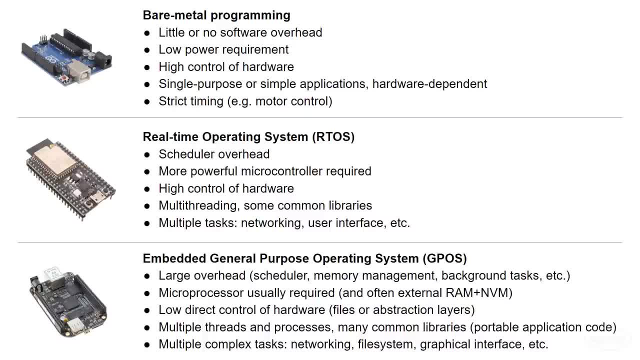 of all this abstraction, you lose out on direct control of hardware and it becomes difficult, if not impossible, to meet strict timing deadlines. You have the option of writing driver code yourself to have better control of connected parts. However, if you want to use embedded OS, you might want to use a different type of OS. 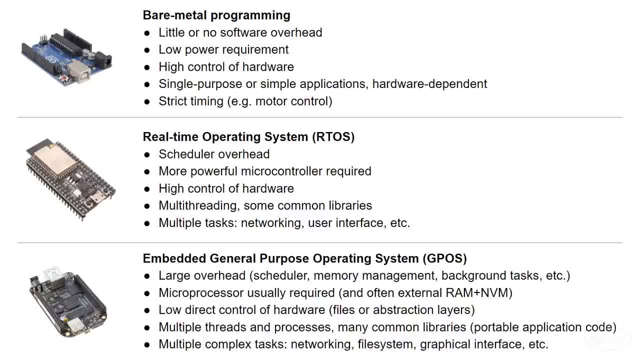 but one of the big reasons to use an embedded OS is so that you can leverage code written by others. Note that real-time operating systems do exist for microprocessor boards like this, to give you better control over the timing of tasks, but you still don't have the same level of precise hardware. 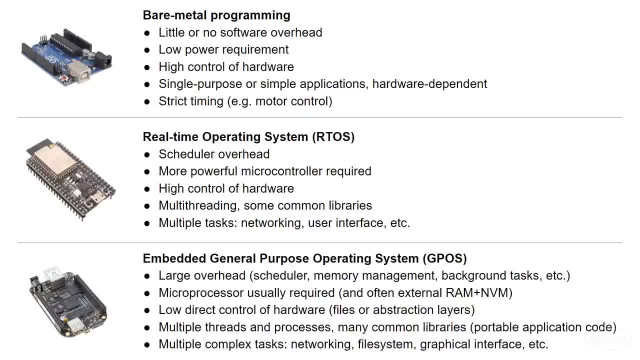 control a microcontroller would give you. As a result, many chip manufacturers include a microcontroller in the same die as their embedded microprocessor. That gives you the best of both: you can run advanced features like networking and complex algorithms on the microprocessor and low-level hardware control and timing on the microcontroller. 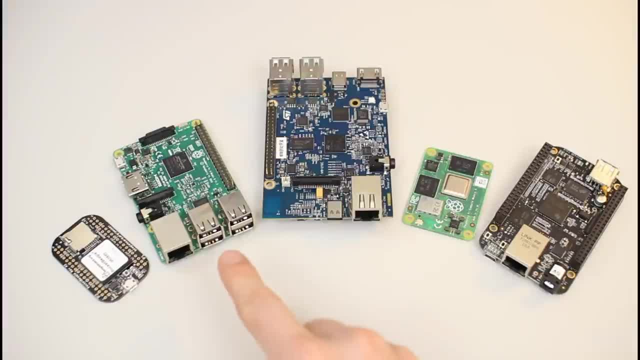 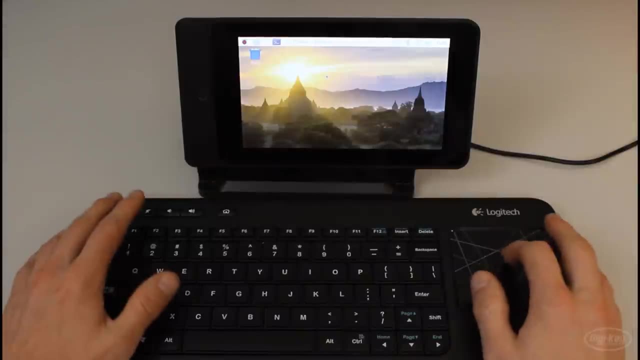 You're probably familiar with the raspberry pi, which is one of, if not the most popular embedded Linux boards in the world. However, it's actually a fairly poor example of how you might use embedded Linux in a professional or industrial setting. It was developed as an educational tool and cheap desktop replacement, and it's 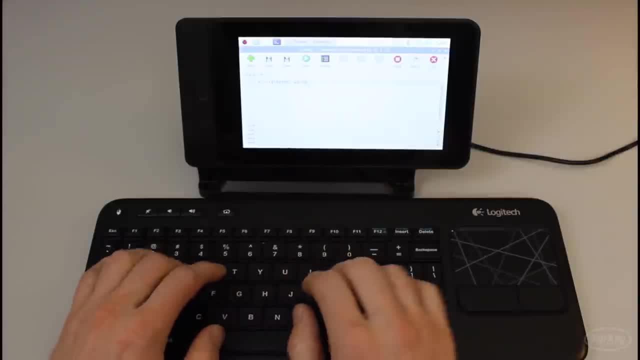 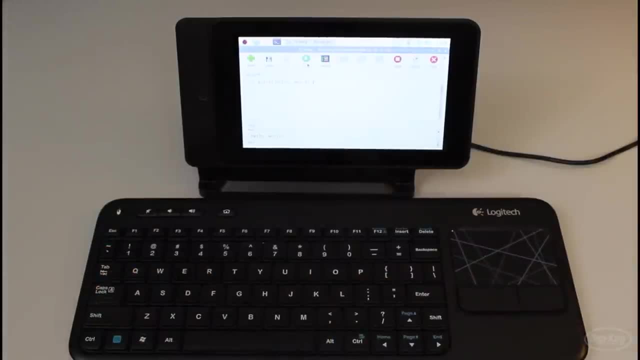 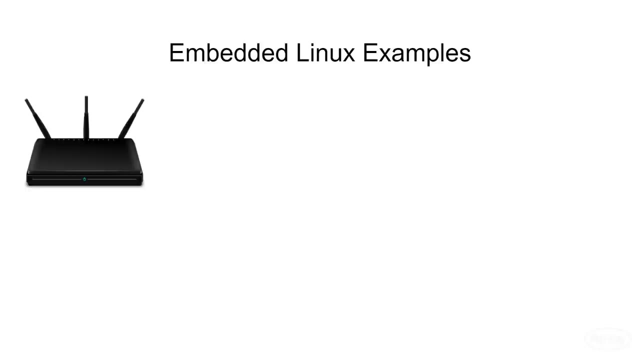 fantastic at doing those things. in fact, due to it having such a high level of support and just working out of the box, i might recommend starting with one to develop prototypes or simply tinker with linux. however, use cases for embedded linux go way beyond just being a replacement for a personal 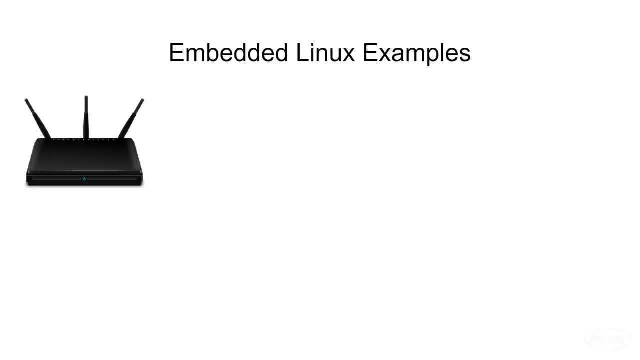 computer. it can be found running things like networking gear such as routers and lightweight servers. you'll also find it in some robotic applications that need to do complex tasks. some rockets and spacecraft, like the spacex falcon 9, rely on linux to run. you'll also find it in some 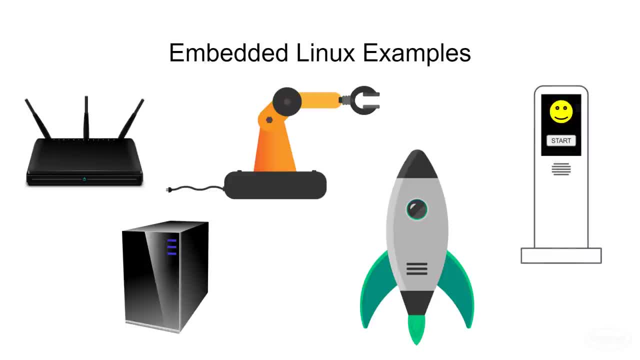 consumer electronics and running the interface in various kiosks. things like networking databases, complex algorithms for something like computer vision, multiple processes and so on dictate the need to use a full operating system like linux over something like an RTOS or bare metal programming. in many of these applications you'll often want a 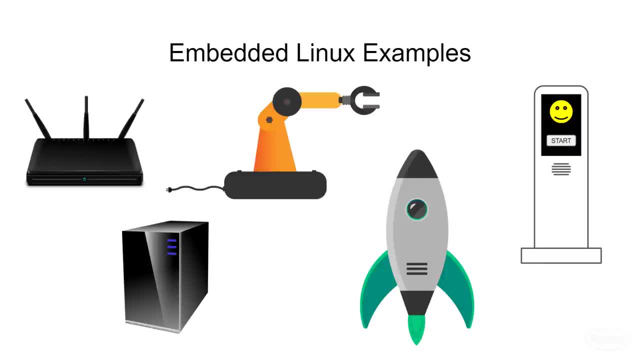 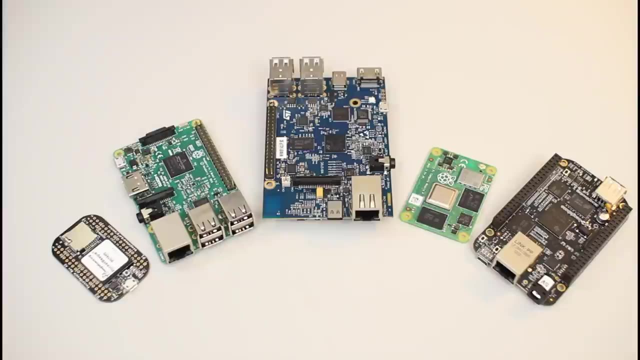 custom operating system in order to save on power and production costs. that means picking the hardware that best suits your needs and running a customized version of linux that doesn't have all the overhead found in something like a common raspberry pi distribution. note that creating your own custom single board computer is extremely difficult. the 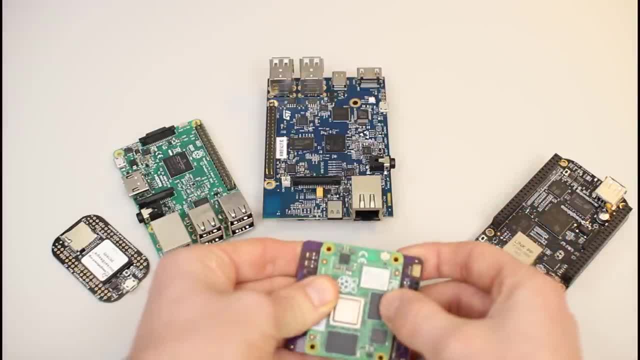 piece of software and software operations you'll be familiar with is what we call bma. i'm using as a user manual, but this is an example. one way to figure out which contents are relevant to your PCB might be complex, but it also means finding or creating drivers for every piece of hardware. 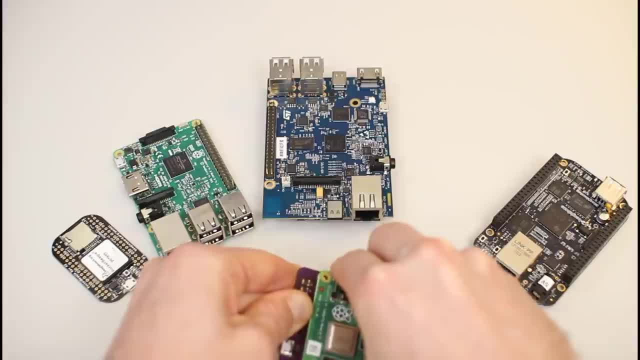 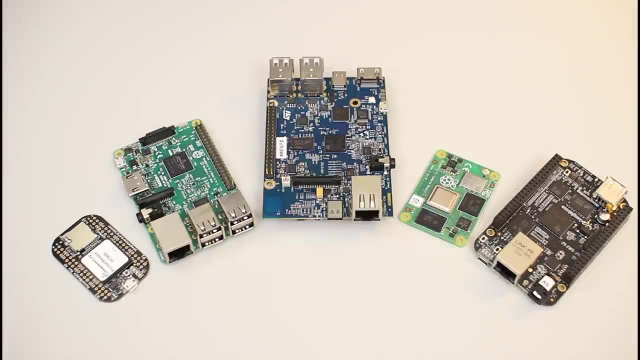 found on the board, like RAM, USB and Wi-Fi. Because of that, some vendors offer reference boards that you can copy, or even systems on a module that you can design a custom carrier board around. What I'm going to show you in this series should work for many popular single board. 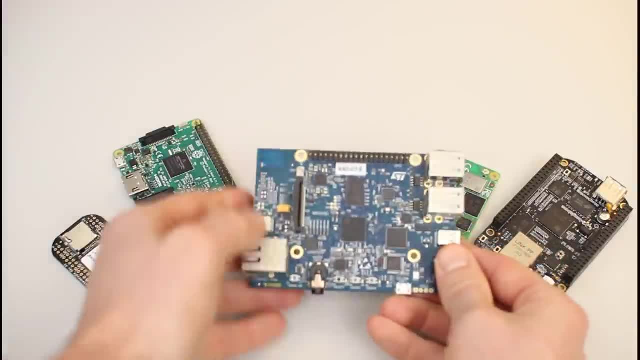 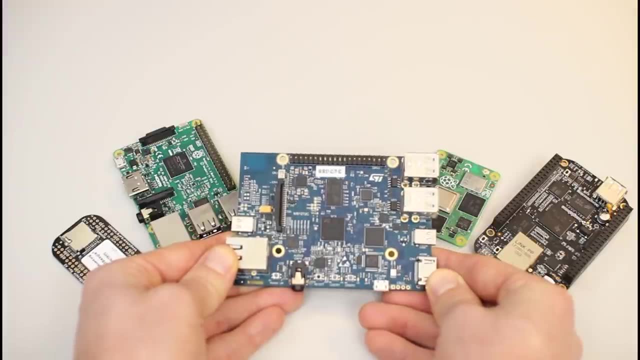 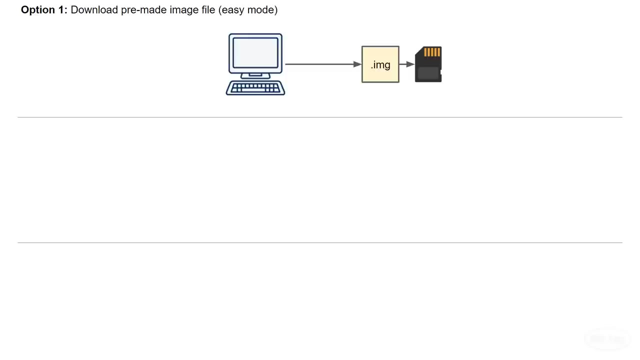 computers and such systems on a module. However, I'm going to focus on the STM32MP157D-DK1 Discovery Kit as an example. If you've worked with a single board computer, you're probably familiar with the simplest method of getting embedded Linux to run, which is where you download a pre-made image file. 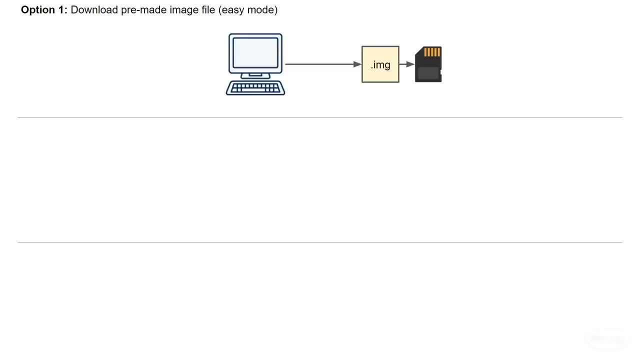 from a website, flash it to your SD card and then plug the SD card into your board. This method is extremely fast and has the best chance of working out of the box. However, it means you have to settle for whatever drivers packages and libraries come with that image. 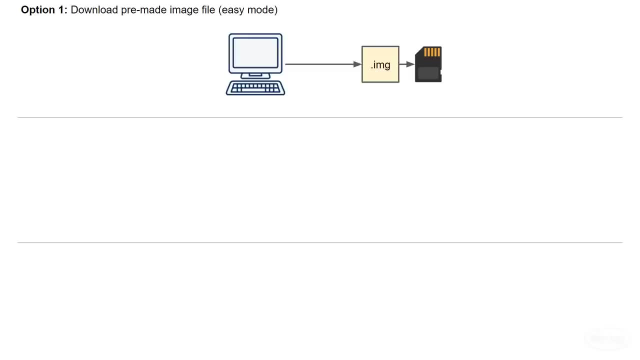 It could mean a lot of bloated software you don't need and that means longer boot times, more flash space used and more power required to run. You could perform customization after flashing, but it would be time intensive if you have to do so for every board that you produce, assuming you're making more than one. 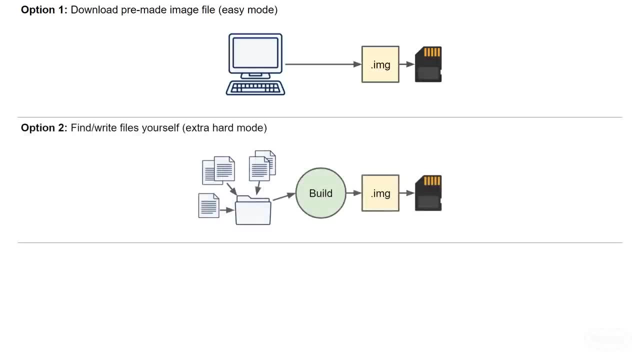 The hardest possible option is to manually find or write the drivers needed to support your board. I would only recommend this method if you are a glutton for punishment. This might mean months of work, putting together source code for dozens or hundreds of drivers and packages and then fighting with compilers. 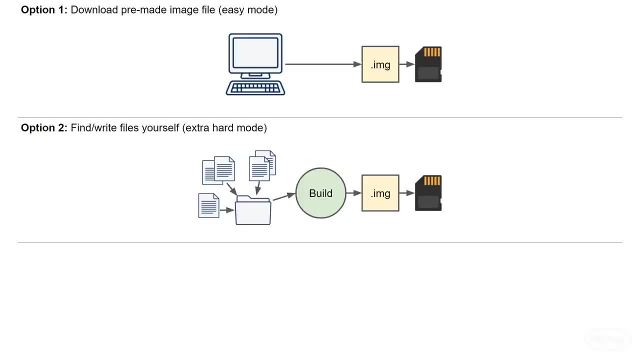 This is probably the biggest reason it's so difficult to design your own single board computer. The third option is to use a tool that helps automate that process. The three most popular tools are probably Buildroot, OpenWRT and the Yocto-Processor. 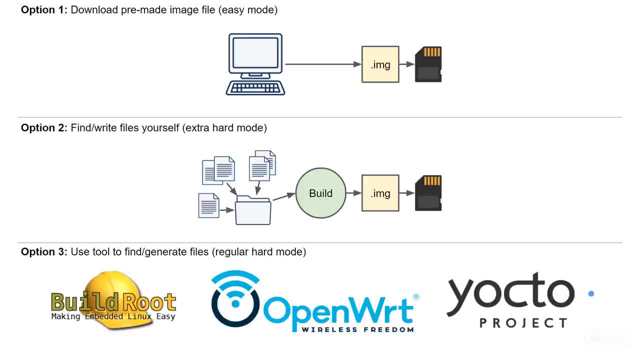 The third option is to use a tool that helps automate that process. The three most popular tools are probably Buildroot, OpenWRT and the Yocto-Processor. The third option is to use a tool that helps automate that process. The third option is to use a tool that helps automate that process. 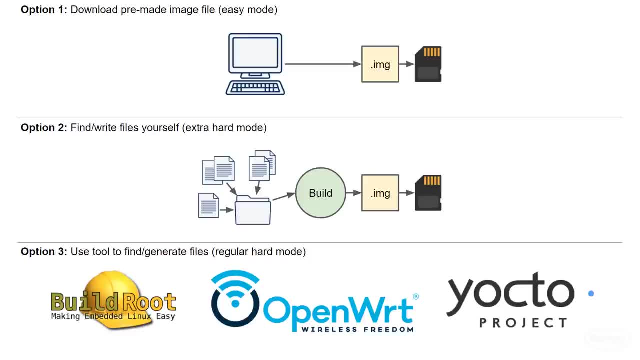 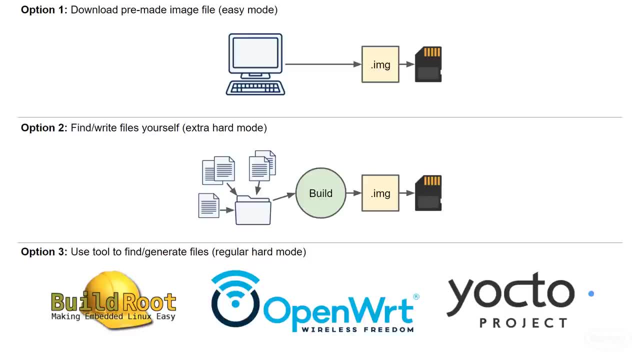 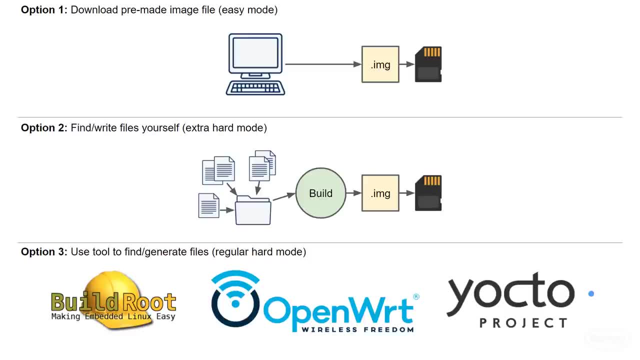 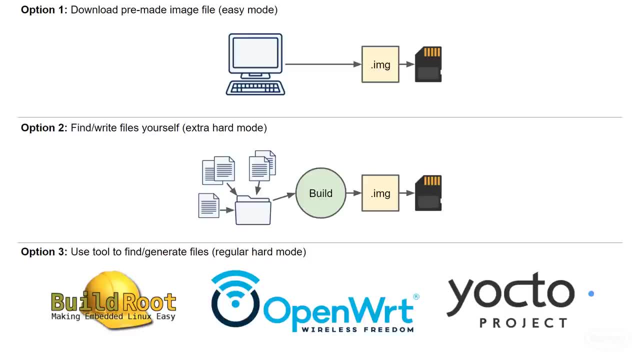 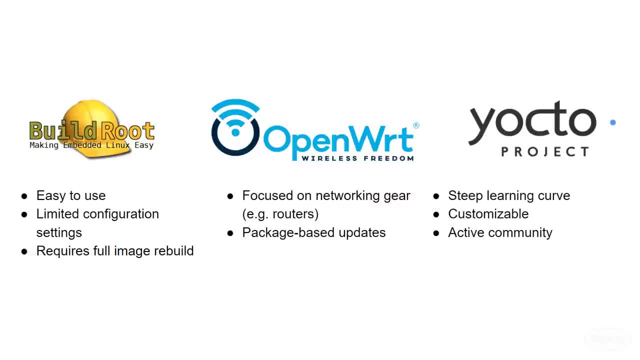 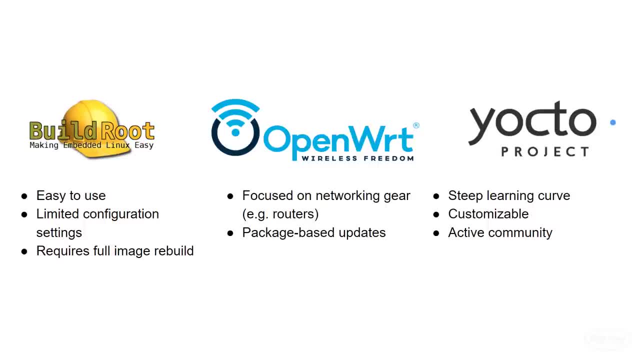 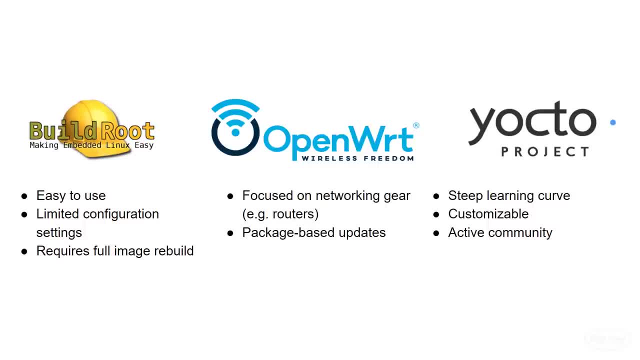 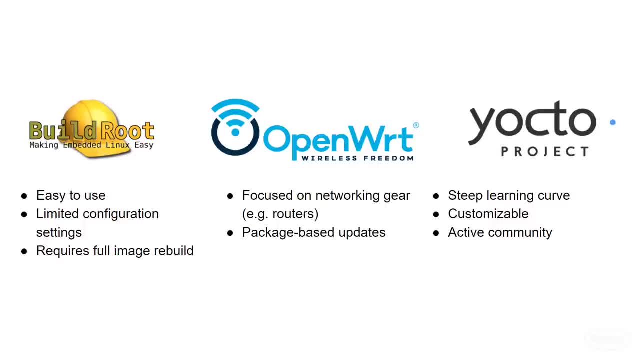 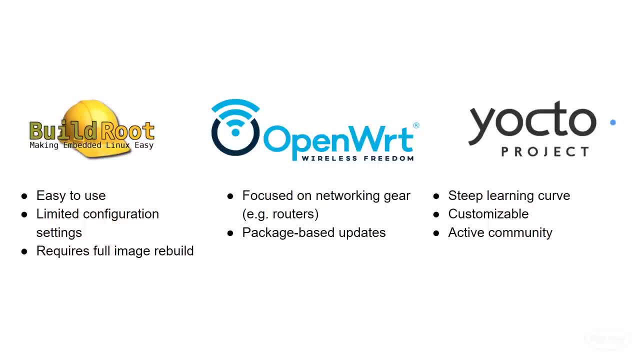 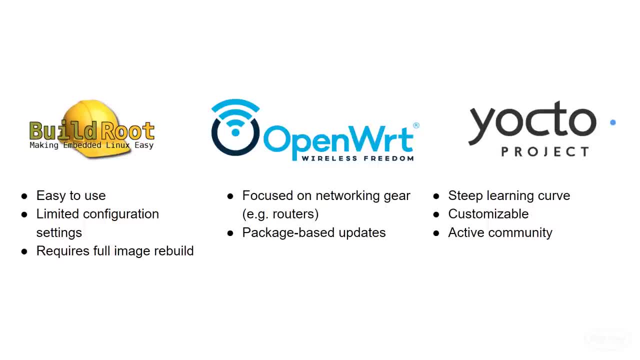 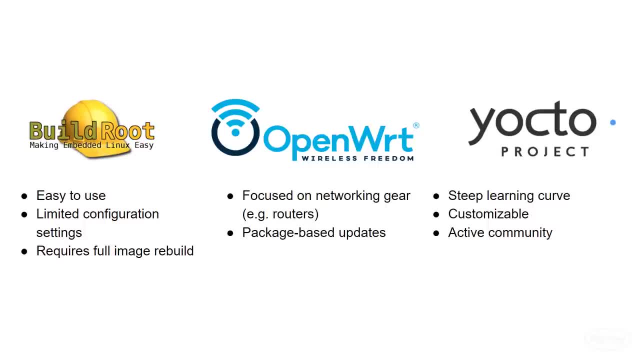 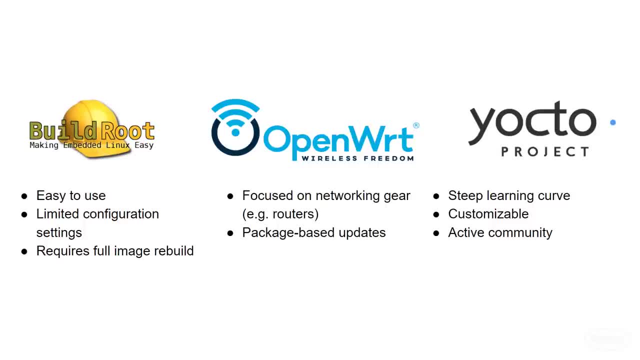 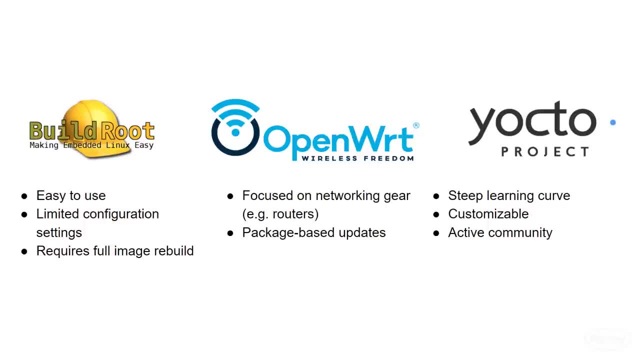 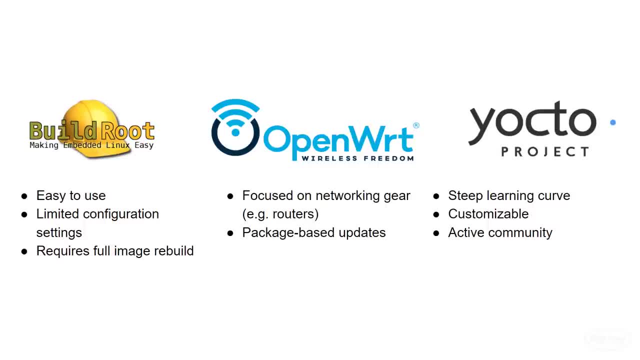 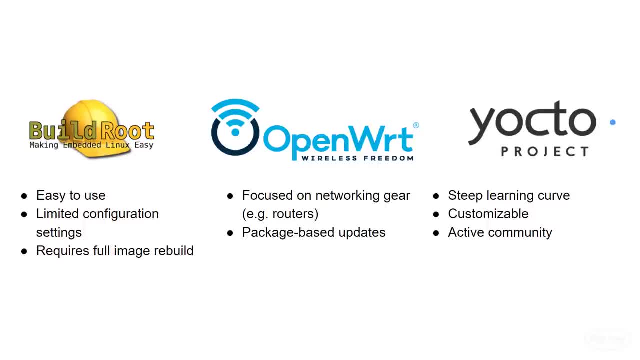 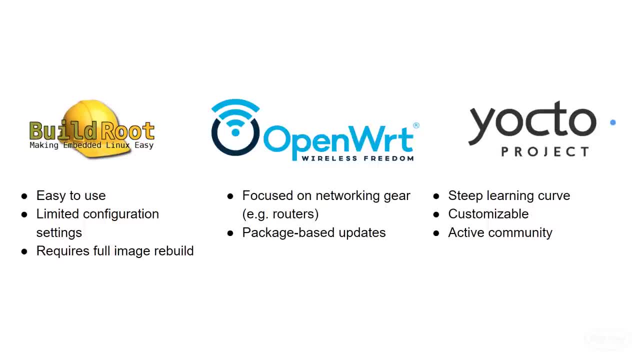 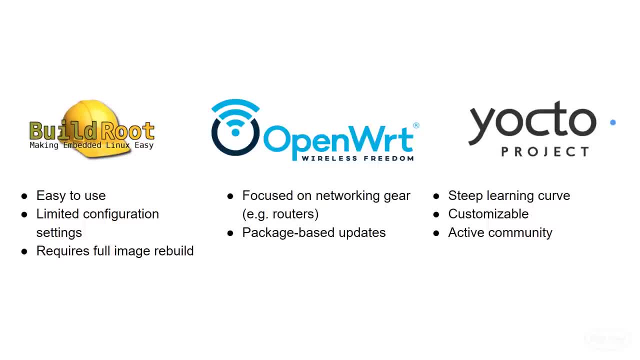 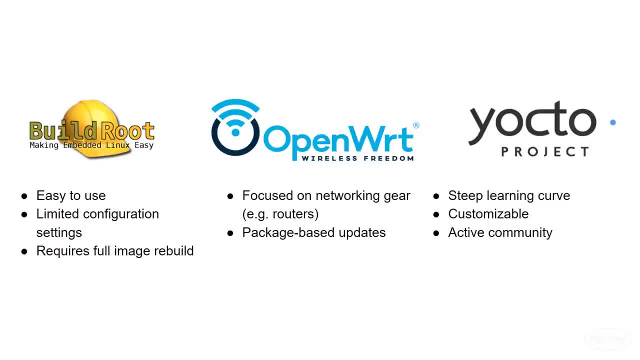 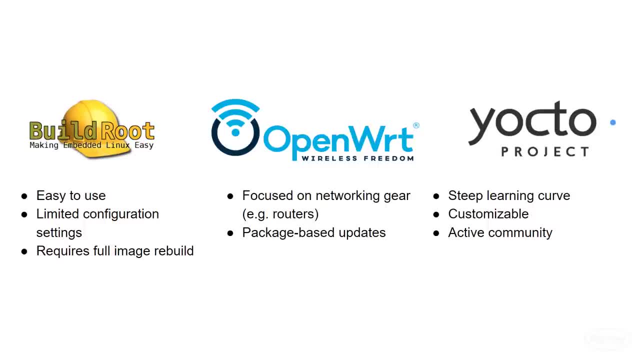 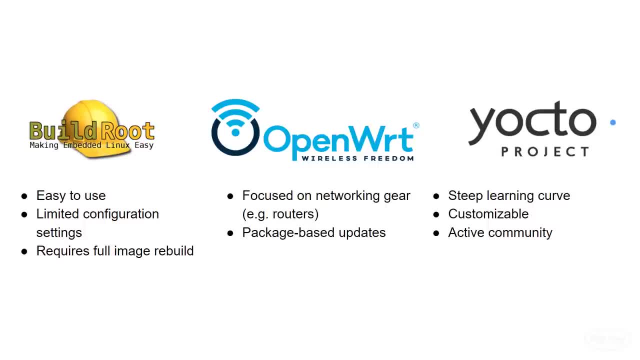 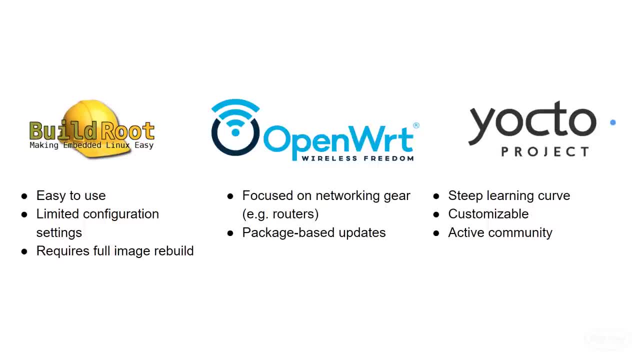 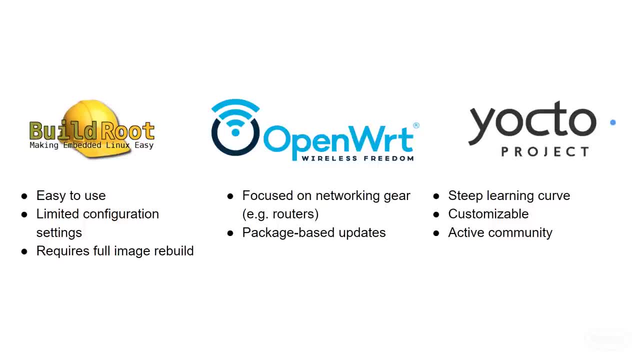 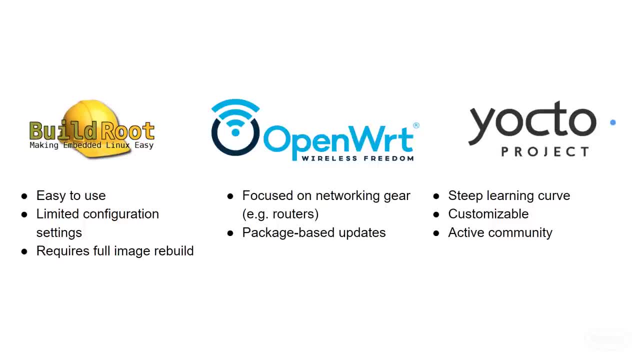 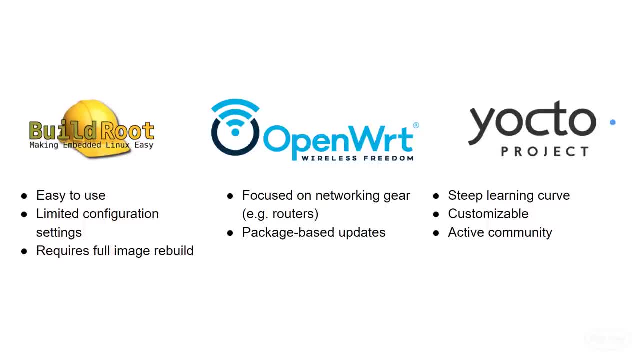 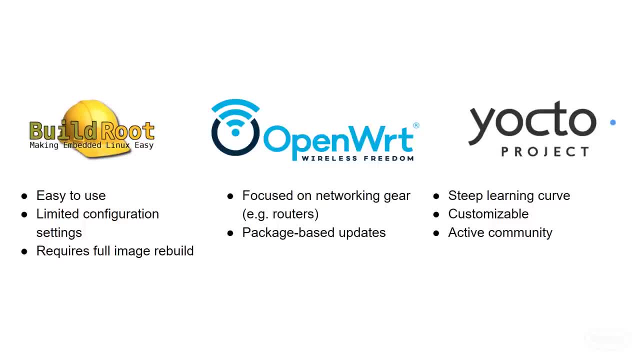 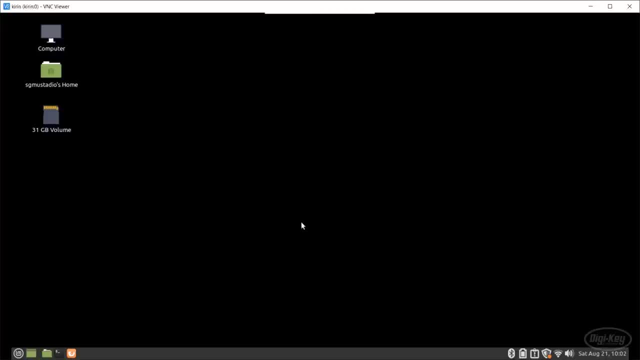 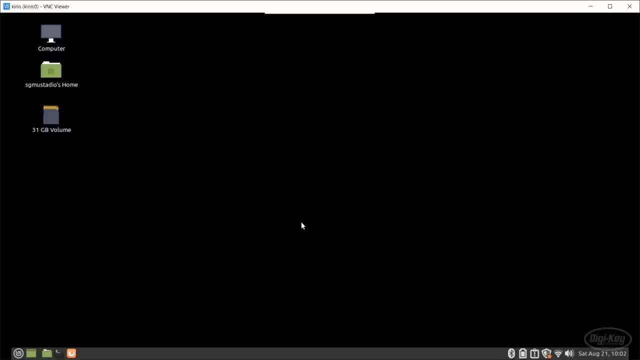 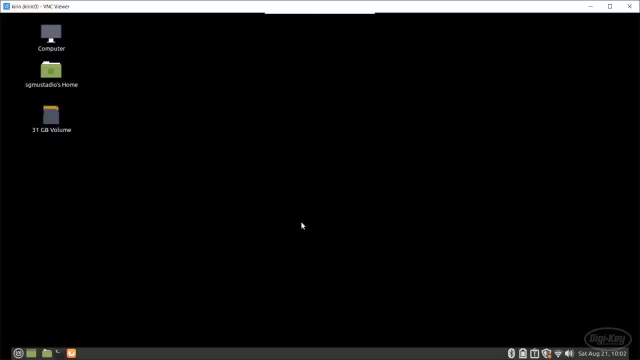 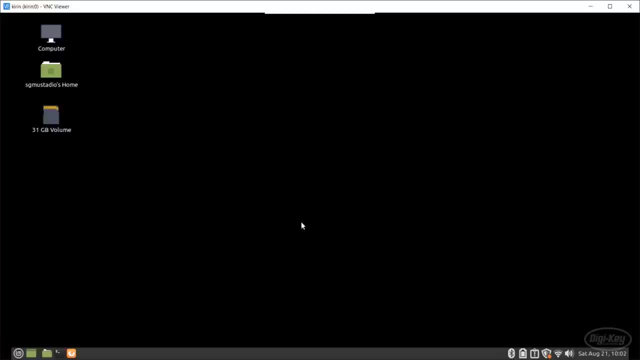 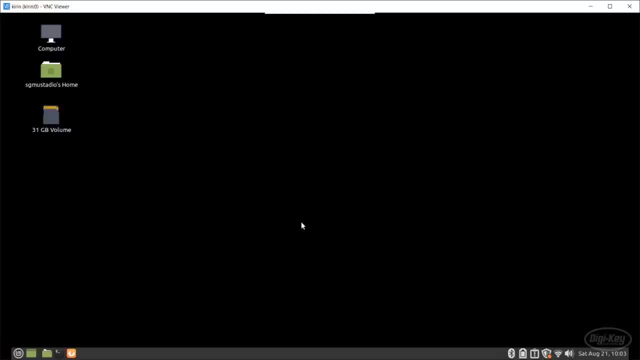 on debian, so a lot of the things that work in ubuntu should also work in linux. mint. i'm doing everything on a separate computer and i've vnc'd in so that i can record my screen. but you're welcome to dual boot your computer. you can set up a virtual machine. there's windows. 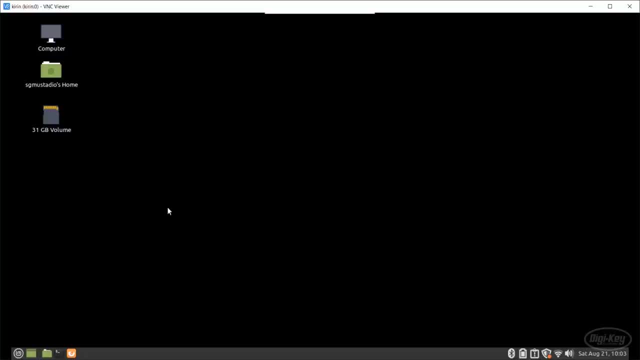 subsystem for linux that may or may not work- i have not tested it- or you can often find a docker image to help you out. once again, i haven't tested it, but i know that there are people out there who have created docker images for things like buildroot and yocto project to begin open up. 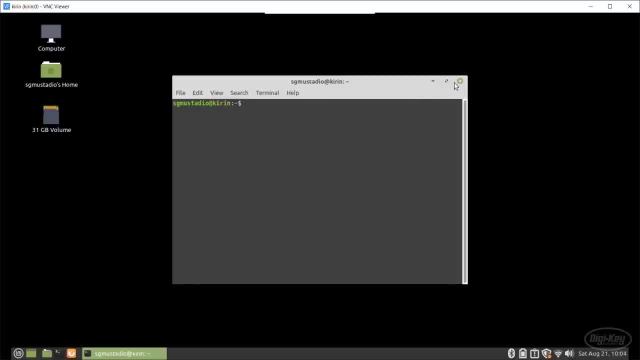 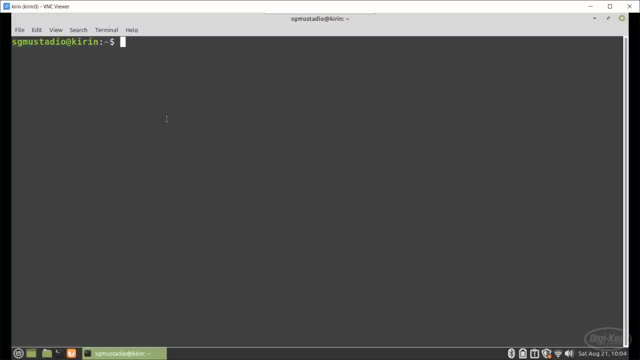 a console. we're going to do almost everything in a console and i'm going to make this a little bit bigger so you can see what i'm doing if you're watching this, say, on a smartphone. for my purposes, i like to do everything in a projects directory. 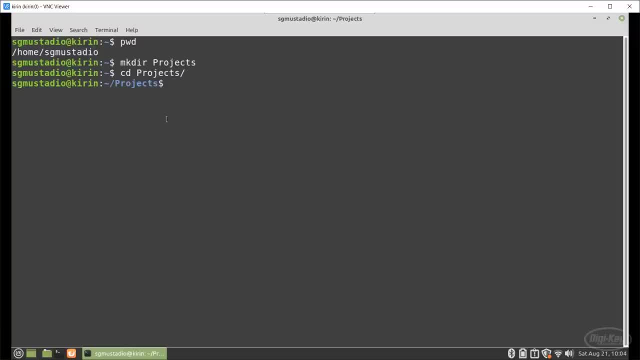 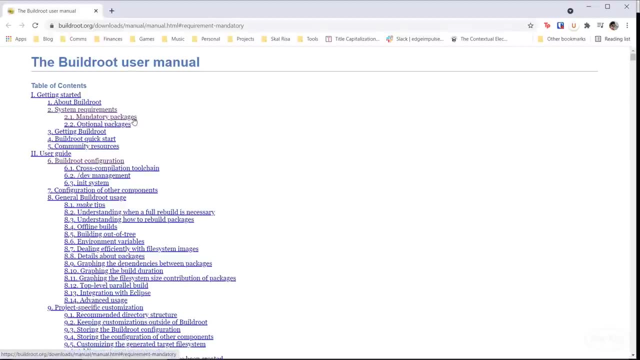 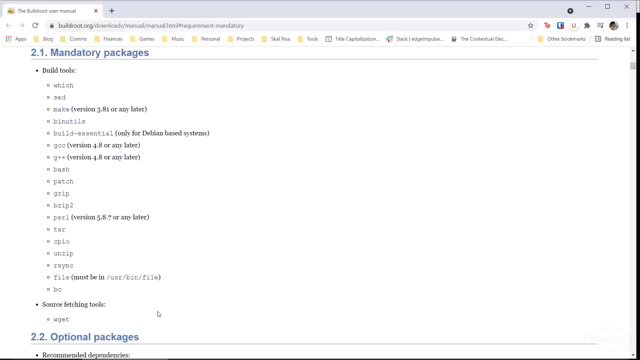 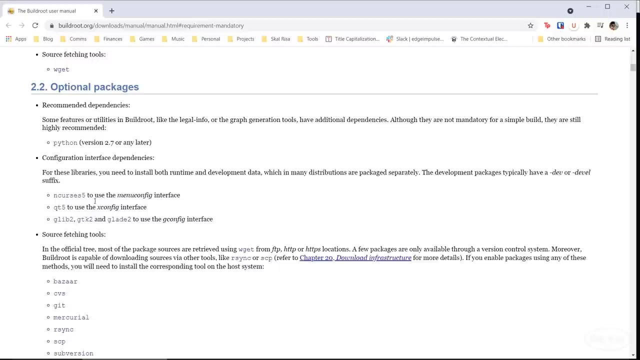 so i will make a project directory and go in there. if you head to the build root user manual, you can find a section on the mandatory packages. many linux distributions come with these packages, but we'll have to install a few extras, especially things like build essential and anchor. 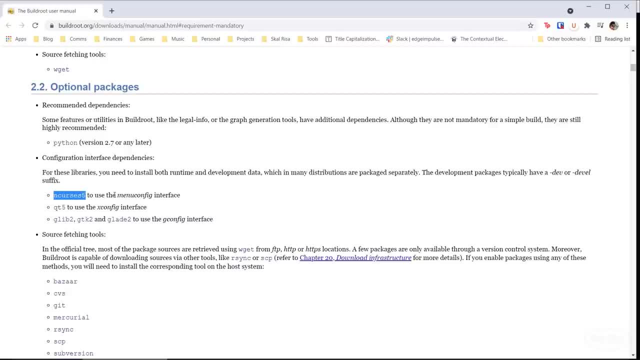 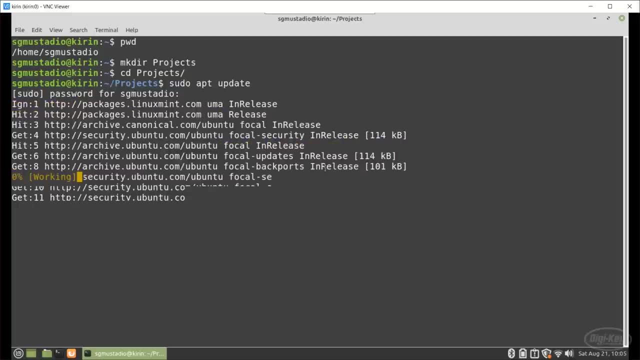 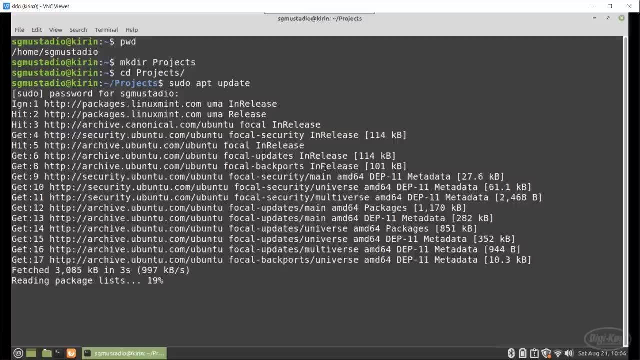 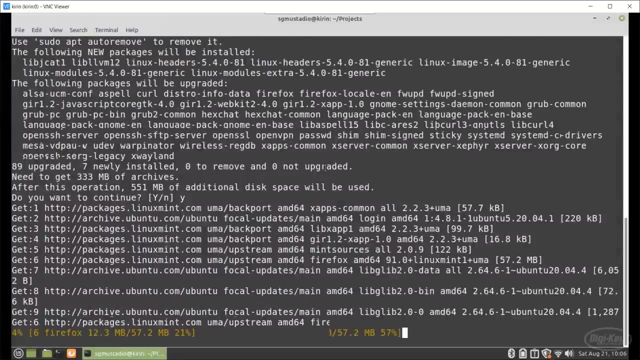 the configuration for a course or a dependent in order to give us a menu config interface which we'll use to configure our build. i always recommend doing an apt update and probably an apt upgrade in order to make sure that you're working with the latest packages. after doing the update, we'll do the upgrade. 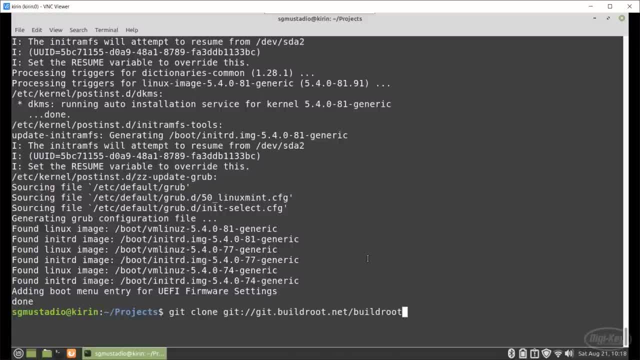 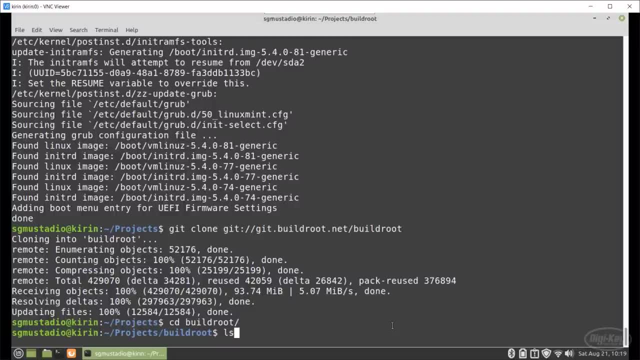 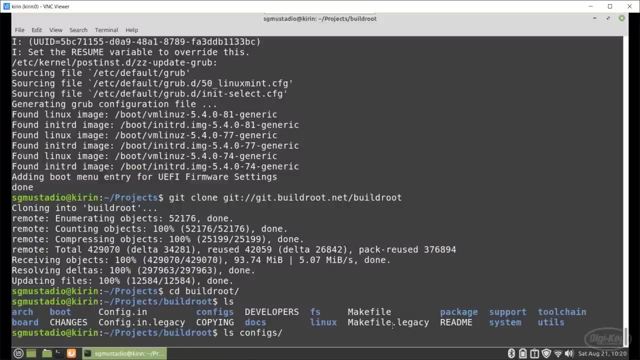 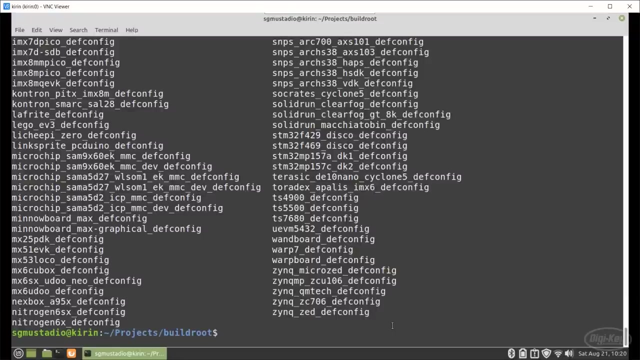 to clone the buildroot project from there. go into the buildroot folder. buildroot has a number of directories. feel free to look through them. the one that we care about is configs, so if we look in there, we can see a number of predefined configuration files for a variety of chips and boards in order to build a linux image. 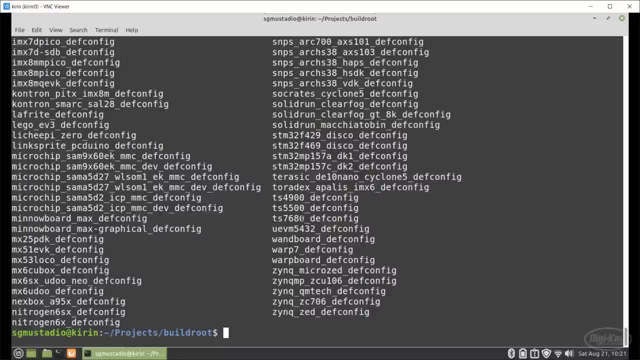 if you don't see your board in here, you can probably look around on the internet to find a buildroot configuration file for your board. i'm using the stm32 mp157d dk1. however, what i found is that this a configuration works well enough at least to get something started. you may want to. 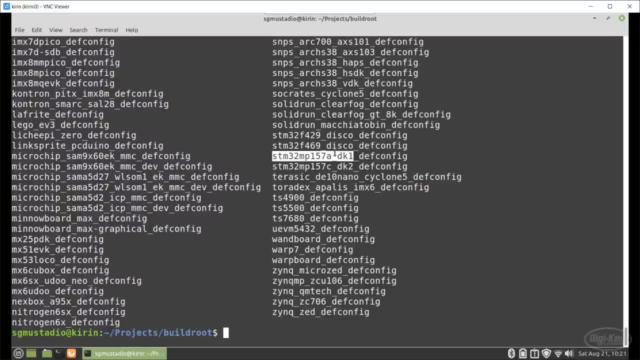 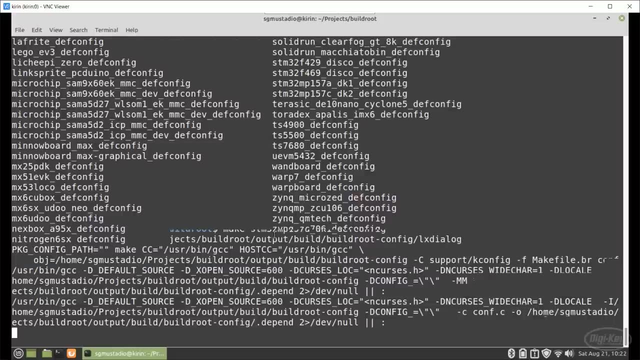 see if you can find a d configuration instead of an a, but let's try this a configuration to see what happens. to do that we just call make and then the name of that config file- defconfig- is default configuration. so we run this, make will read it and construct a dot config file. 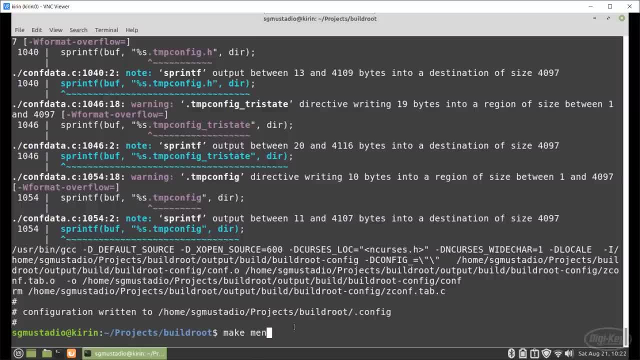 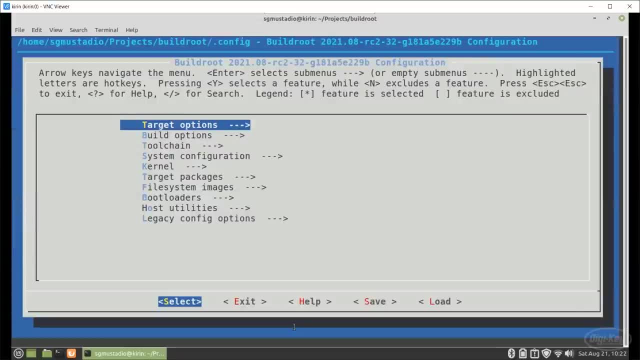 in the buildroot project. from here, we can call make menu config, which will read in that configuration file, and then bring up a sort of graphical interface in order to adjust the options for our build. feel free to look through these. this is how you would make changes to things like your kernel. 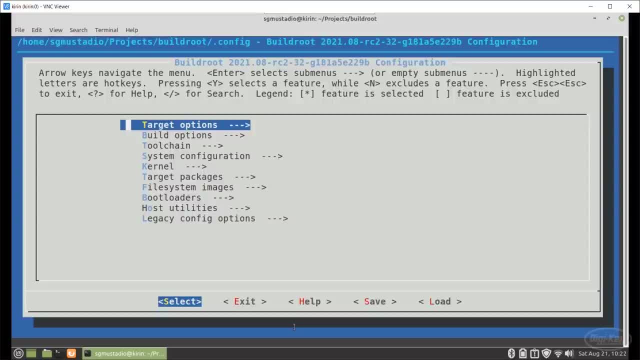 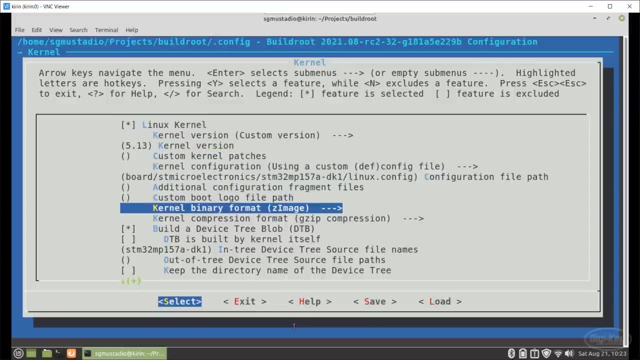 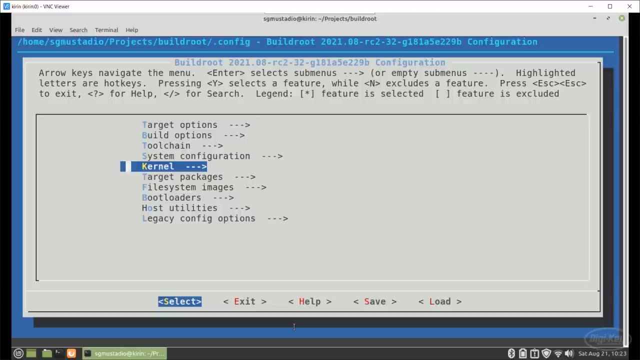 or adding packages prior to building the linux image. in fact, i can go to kernel and you can see the various kernel options that you have available here. we won't be exploring these right now, so use your arrow keys left and right to highlight exit, press enter and then select exit again and hit enter to exit the whole menu. config, the default configuration. 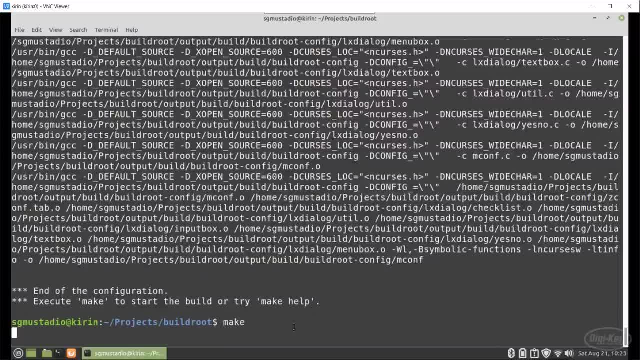 should be good enough from here. all you need to do is type make and you let this process run for a while. this could take one or more hours in order to build the linux image. so i recommend going to make a sandwich or grab a cup of coffee or go do something else while this builds. but you want. 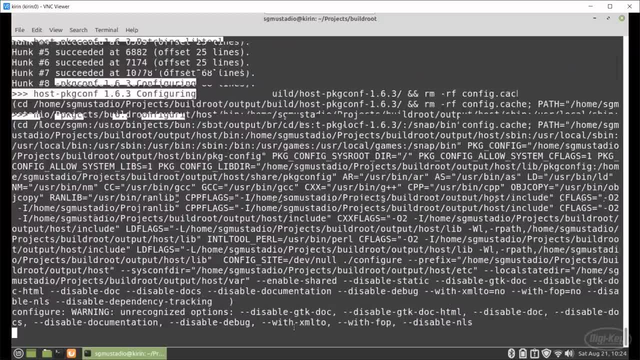 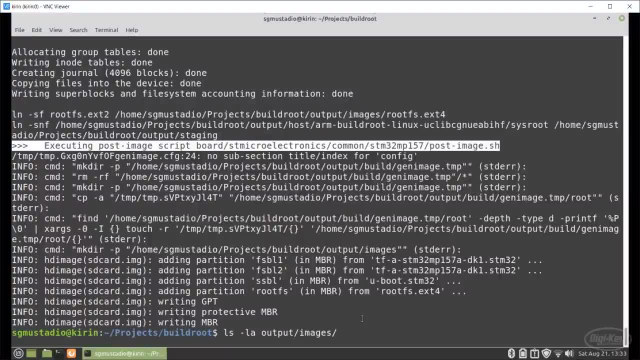 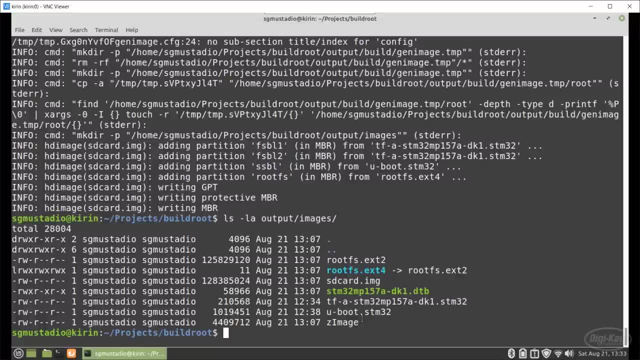 to keep an eye on it to look out for any errors that might appear. once that process is done, you can look for the output of buildroot in output images. here you should see a number of potential image files, or maybe even a collection of files that you would copy onto your boot and root file. 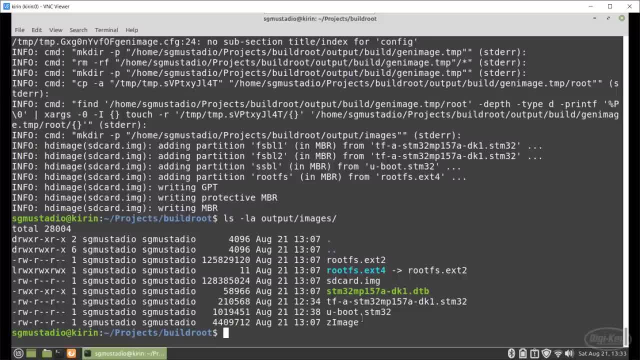 systems. in this instance we have an sd card dot img file that we can just copy directly to an sd card bit for bit using a tool like dd to create that linux image and let that buffer. while this is up and running image for us, I'm going to plug an SD card into an SD card reader on my computer and you can see here. 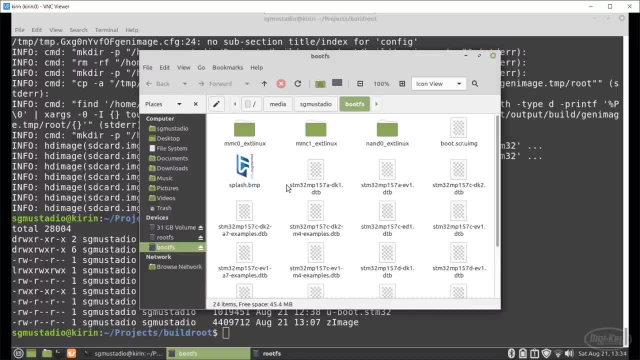 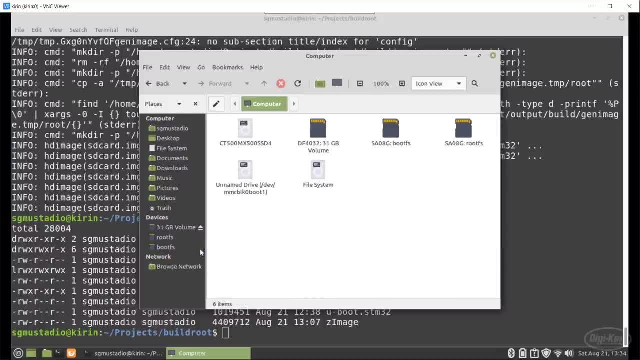 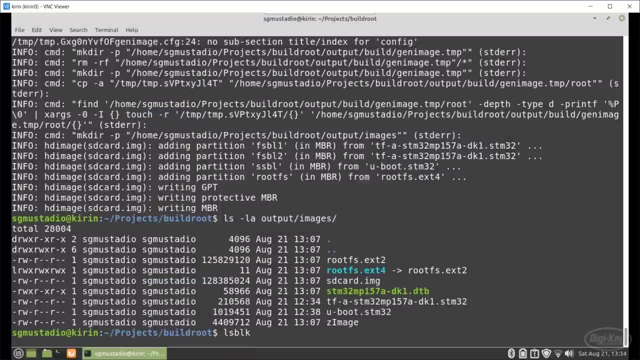 that it auto enumerates using some other image that I had there previously. We need to unmount these partitions, so feel free to use the you mount tool on the command line or just use a graphical interface like I do here. From there, type lsblk for list block and that's going to show our various storage devices. 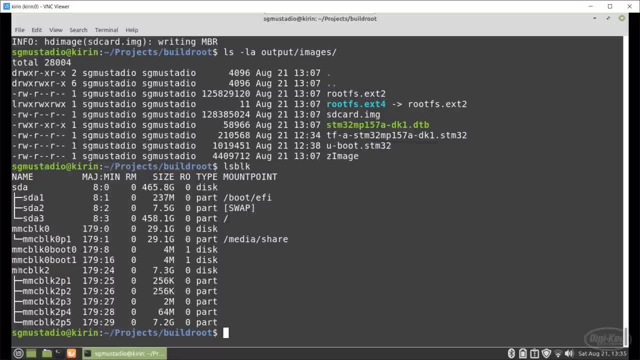 I just plugged in an 8 gigabyte SD card so it looks like it's on MMC block 2.. The SD card image file contains all of the partitions needed for our Linux image, so we just need to do, a bit for bit, transfer directly to the raw device. so we're not going to worry. 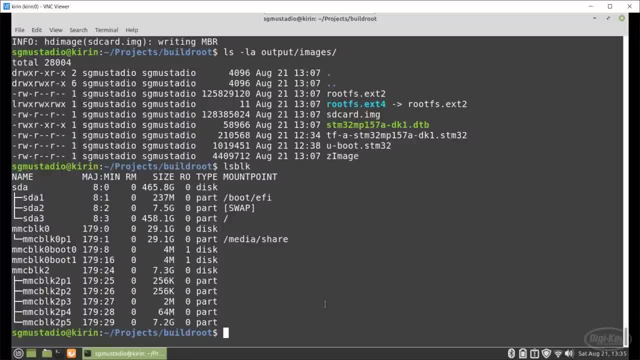 about the partitions here. In fact, we're about to delete them In this process. we'll use the dd tool to do this bit for bit copying. I need root privileges to make it happen, so I'll call it with the sudo command, and if is the input file that we're going to be copying of is where we want to copy it to. 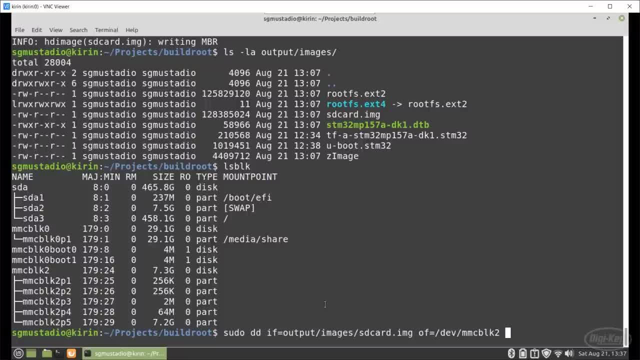 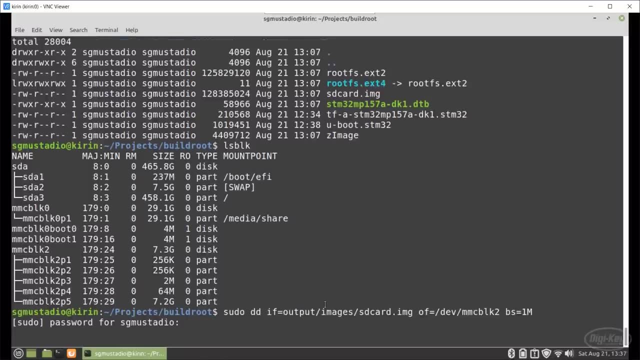 So I'm going to point that at MMC, block 2.. We can also set the block size, And something like one megabyte is probably fine. it just speeds up the copying process. I'll put my password in and let it copy By default. dd does not output any sort of status, so you just kind of have to take a. 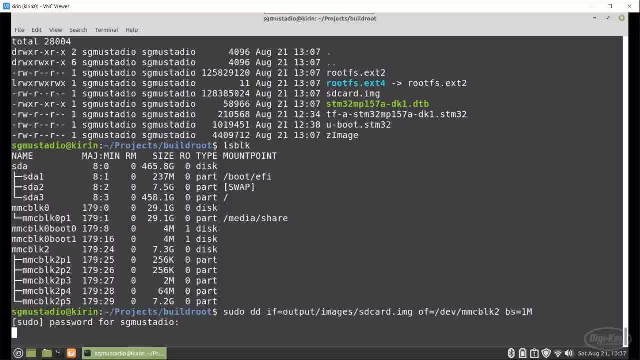 leap of faith that copying is happening, And in this case there are a few hundred megabytes that need to be copied, So this might take a few minutes. When it's done, dd should tell you that everything was copied and that there weren't any errors. 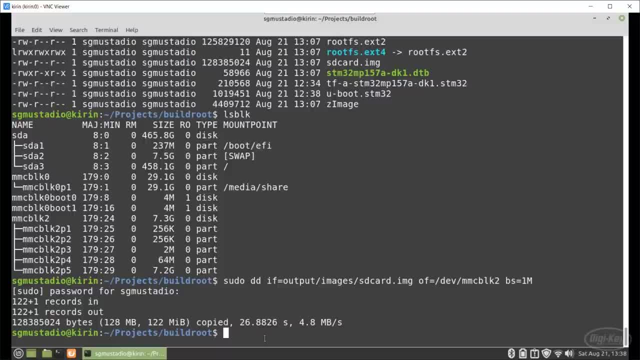 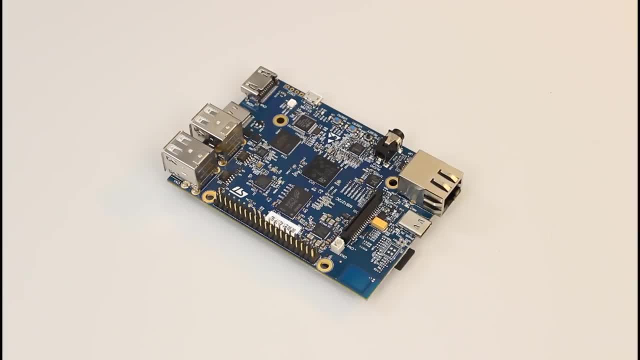 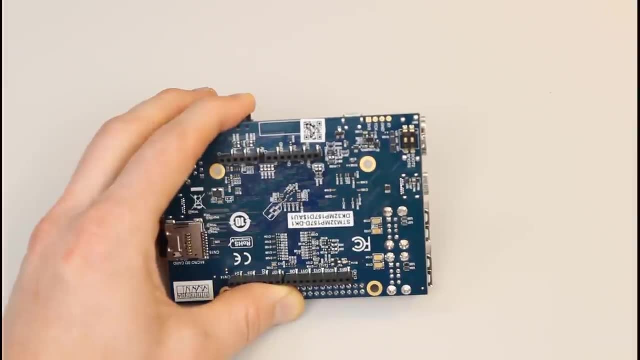 Now all we have to do is remove the card from our computer and plug it into our board to see if it works. Plug the SD card into the board. for this particular board you'll want to flip the boot zero and boot two switches to on in order to have it boot from the SD card- almost all embedded. 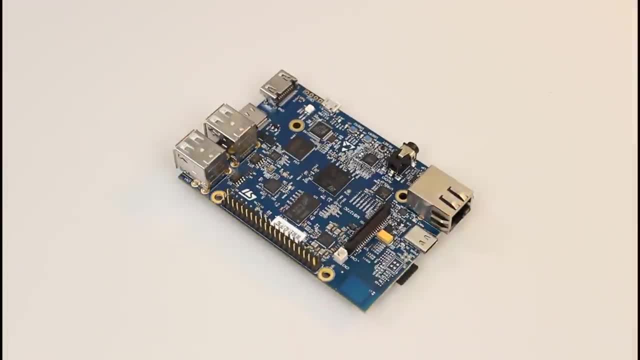 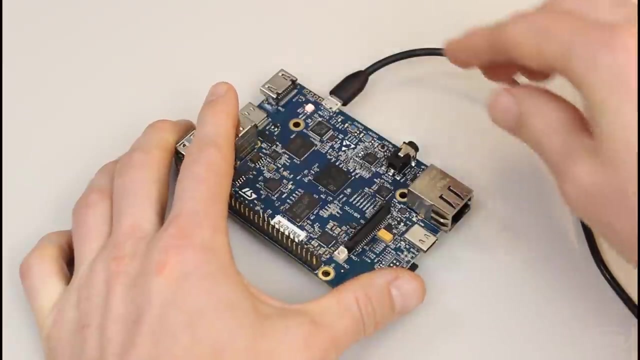 Linux boards will have a serial port dedicated to providing a console. on this particular board You are To the onboard ST link debugger which also does USB to serial translation by default. the configuration file has you are for being used as the console port, So we can just plug a USB micro cable into the ST link port and connect the other end. 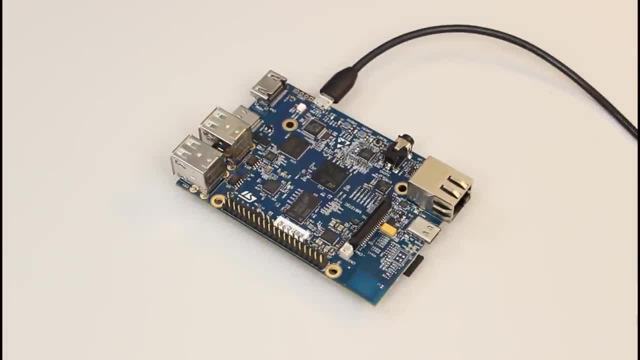 to our computer. If your board does not have an onboard USB to serial translator, you'll likely have to figure out which you are port the console is on and then connect a separate translator. like this, You can also plug a USB cable into the ST link port and connect it to your board, which. 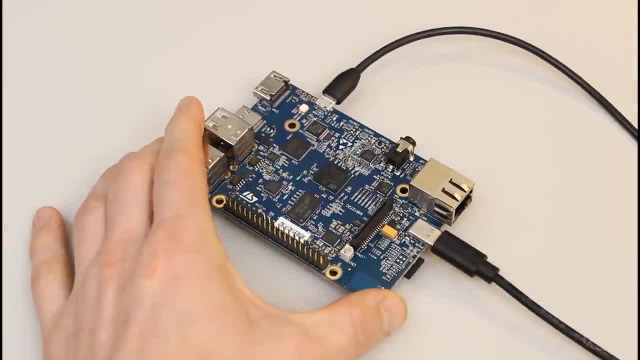 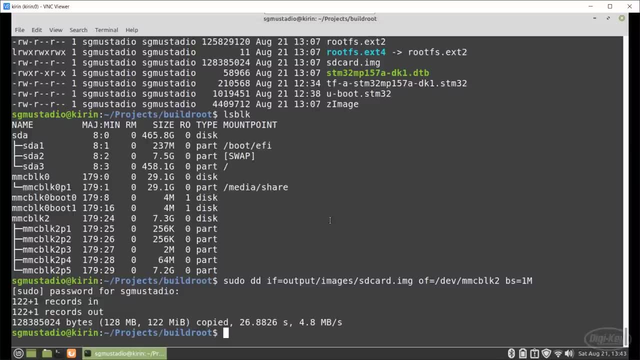 for me is a USB C cable that's plugged into a 5 volt, 3 amp supply. To get the serial console from our board you'll need to install some sort of serial terminal program on Linux. This is probably something like screen or mini com. 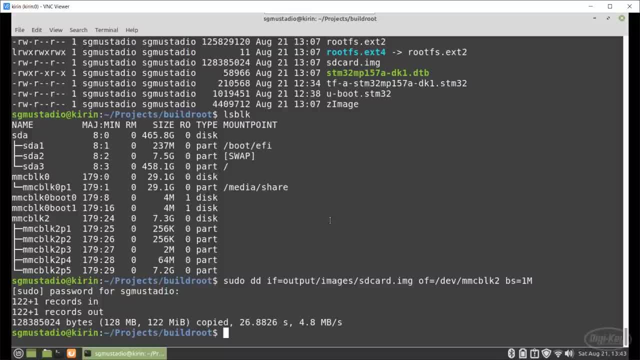 I'm a big fan of Pico com because it's really simple. If you don't have it, feel free to install it with whatever package manager you're using. If you don't have it, feel free to install it with whatever package manager you're. 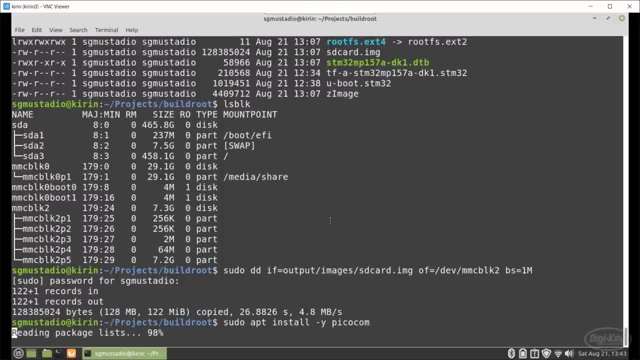 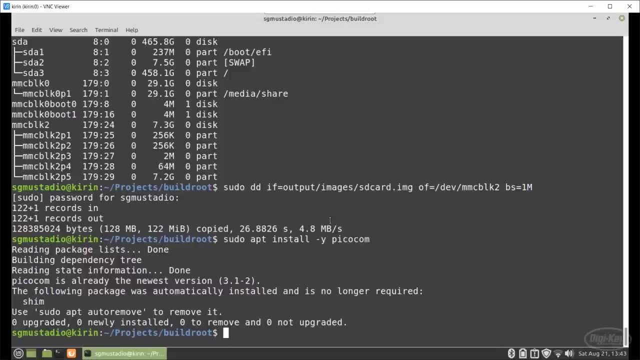 using It's already installed. for me, The one thing that I noticed about Pico com is that you need to add your current user to the dial out group in order to get it to work. Otherwise, you might get a permission denied, even using it with sudo. 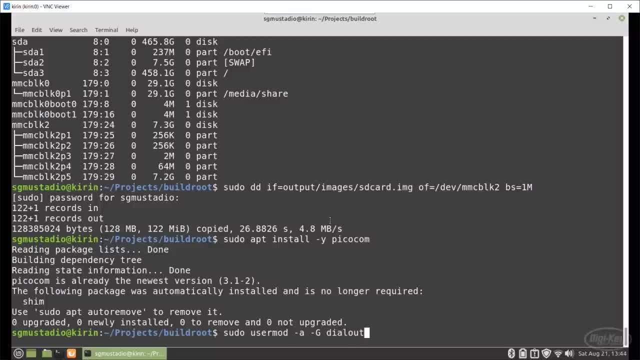 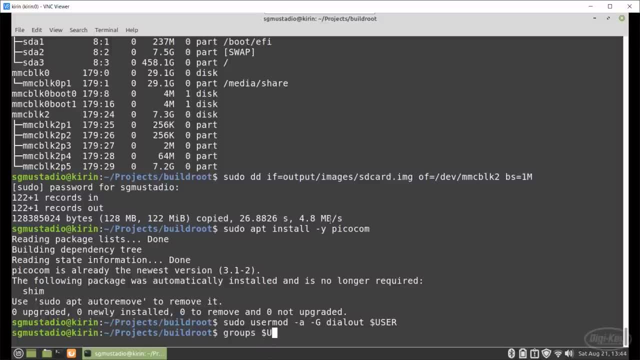 So to correct that we can just call user mod And then Connect the current user to the dial out group and we can check to make sure that dial out appears as a group for our user by using the command groups From here. you just call Pico com, give it the baud rate with dash B and then tell it what. 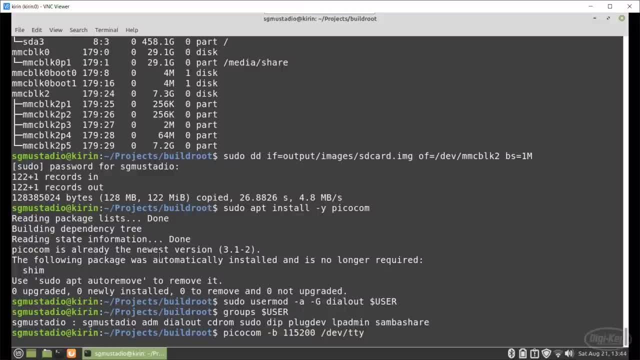 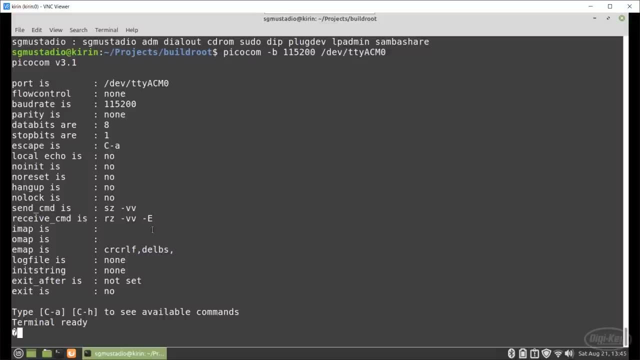 device is connected to your single board computer. For my case it's TTY ACM zero, but that might be something different for you, depending on your particular version of Linux. I'm going to connect it And You might have something or nothing here, depending. after all of this information is printed about. 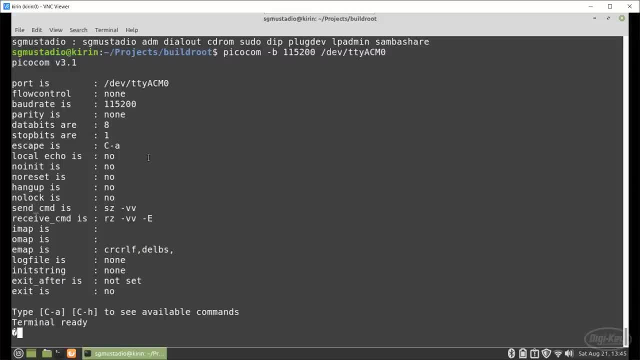 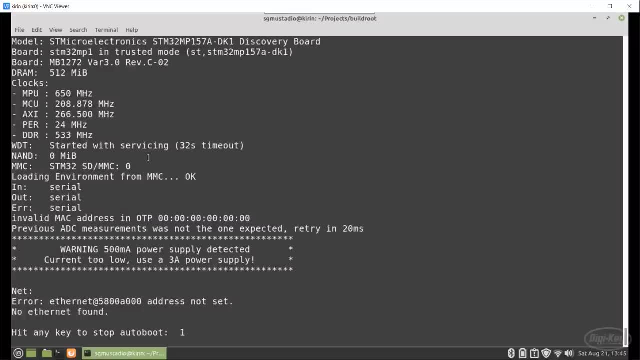 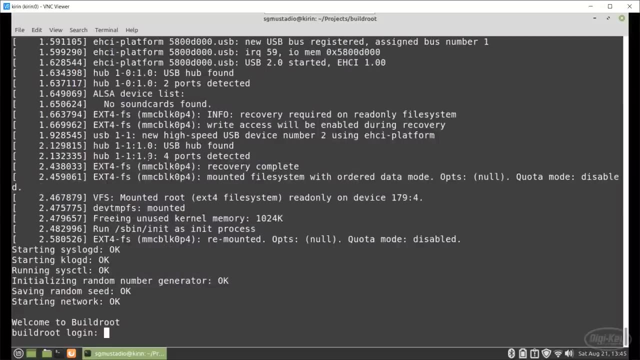 the connection. What I like to do is hit the reset button on my board or cycle power, Which will cause all of the boot messages to appear and you can watch what's going on with the various boot processes. There are several boot loaders that need to happen and we'll talk about those in a later. 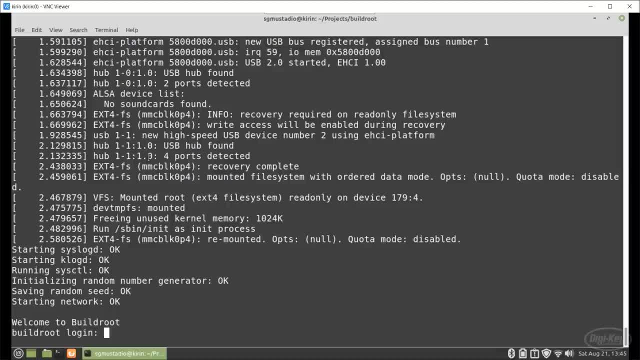 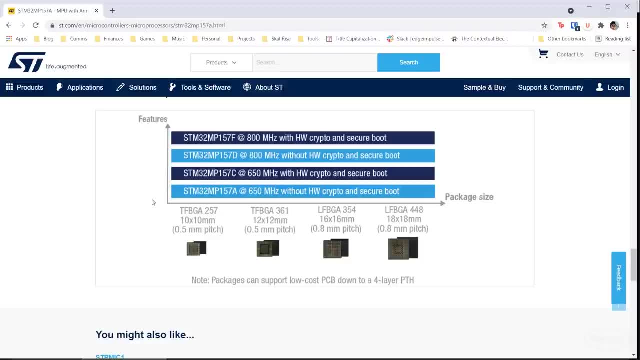 episode, But For now, What we care about Is that we have a login prompt. That means Everything worked During the buildroot compilation process. I looked up the difference between a 157D and a 157A. 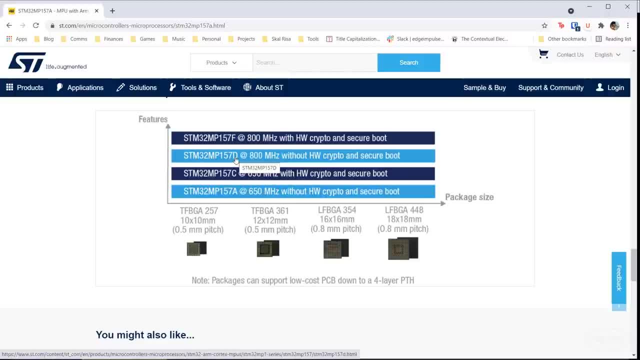 My board is the STM32MP157D that supposedly runs at 800 megahertz, whereas the 157A runs at 650 megahertz. I'm kind of surprised this works, but it happens to work anyway. The buildroot configuration likely tells the clocks to start up. 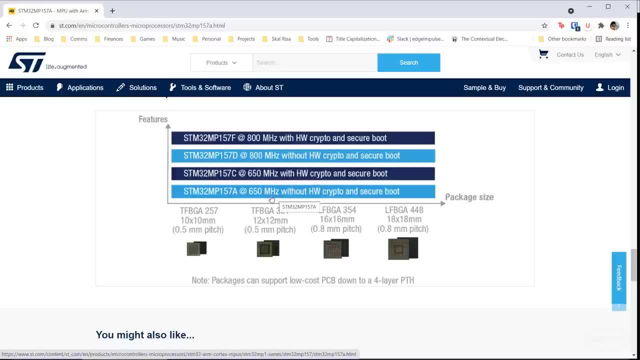 At 650 megahertz, which means that I'm probably just underclocking my board a little bit, which is fine for this experimentation. but if you were going to use buildroot for your processes, I highly recommend finding a configuration file that works for your particular board. 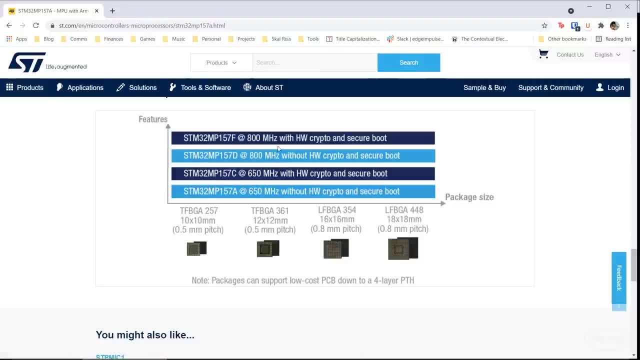 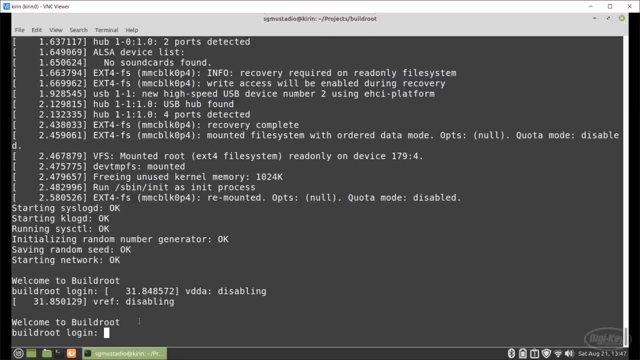 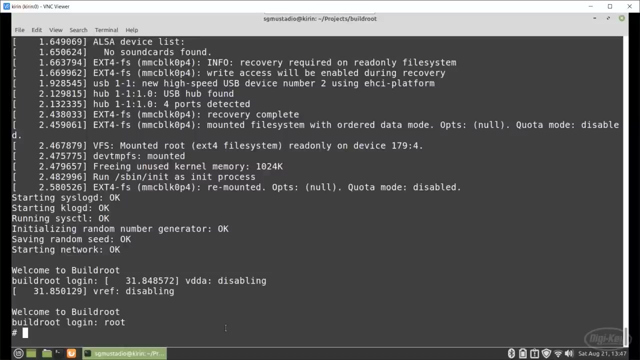 and your particular chip to make sure that you're not missing out on things like clock cycles. Now that I have everything here, I get my login prompt And for a very basic buildroot image, the login is root and there is no password. So we are in Linux right now, running on the single board computer. 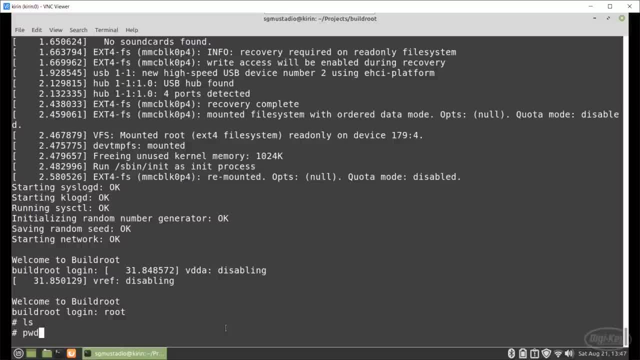 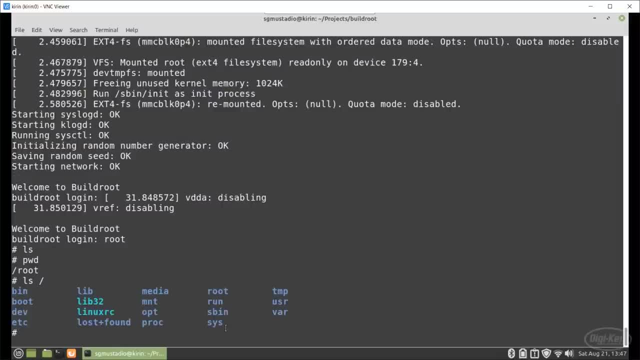 If I take a look at any files, nothing here. I can look at my current directory. that's because I'm in root and I can see what is in the root directory and you can see it's pretty normal Linux stuff. but there's just not much here. there's no user, there's really. 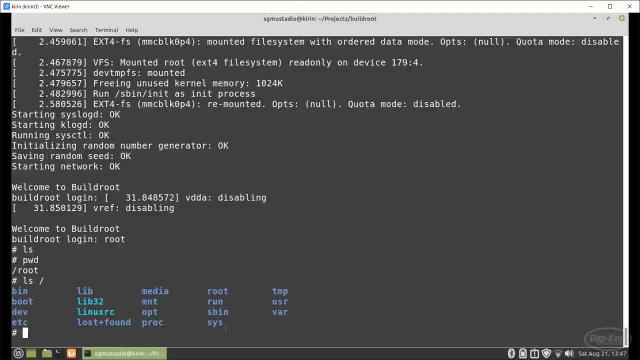 no packages. This is as basic as it gets. You'll probably find that there's no package manager. It's really hard to install stuff unless you bring in cross compiled binaries. So if you want to GCC, you'd have to cross compile it and bring it in and then build. 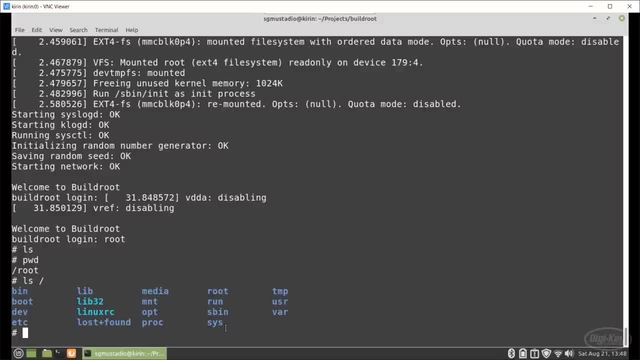 your own programs on this board, But a lot of times what you'll find is: you don't want to do that. you want to develop applications on your host computer, test them and then bring in the binaries to your deployed image file, Just because development is faster and it allows you to make an image that can be copied. 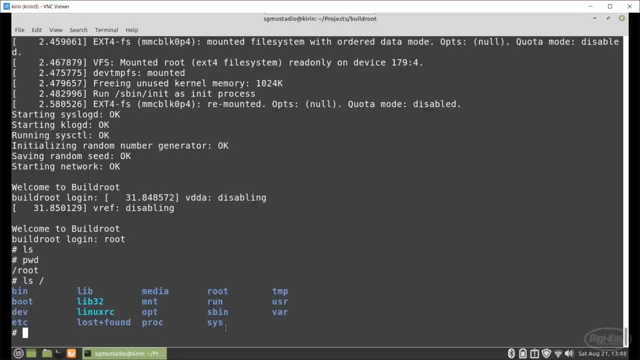 to production, copied to any number of devices that you want. We'll explore development later, but for now let's do a very quick script to see that this is indeed running. Most of these images come with VI as a very basic editor, and I'm going to create a simple. 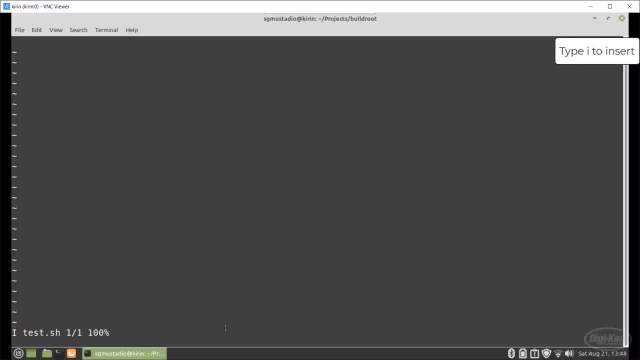 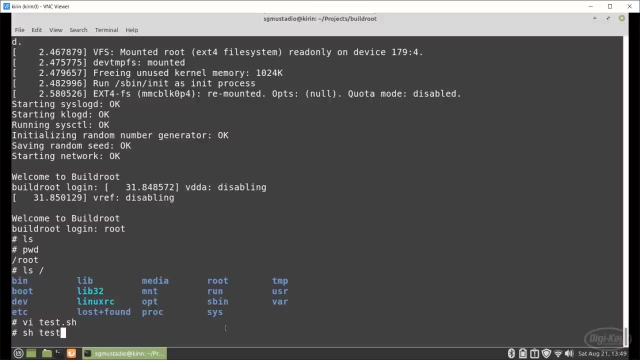 script here In VI. I'm going to push I to insert And I'm going to echo something really basic to the console. Press escape to get out of editing mode and then type colon WQ for write and quit. Then we can test this script by running testsh and it should print something to the console. 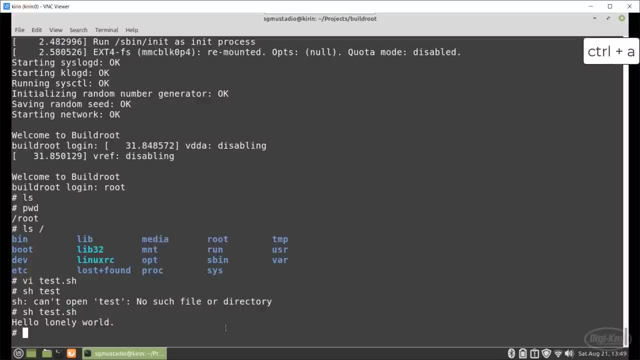 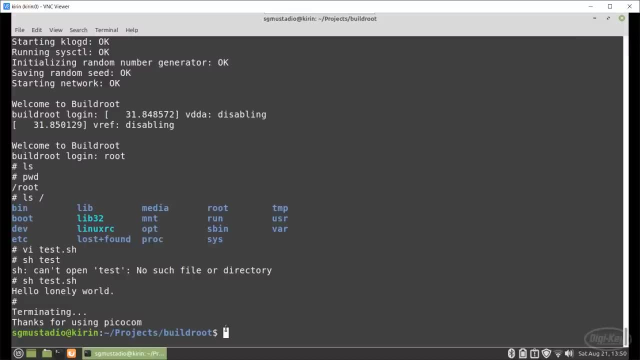 When you are done with picocom, You can press control A And then control X to give it the command that you'd like to exit out of picocom. I hope this gives you a good demonstration for how to create your own Linux image and.